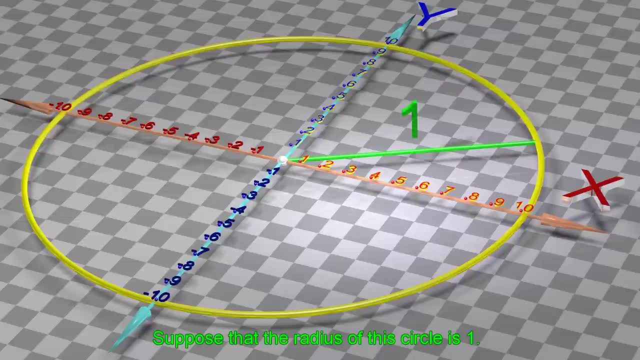 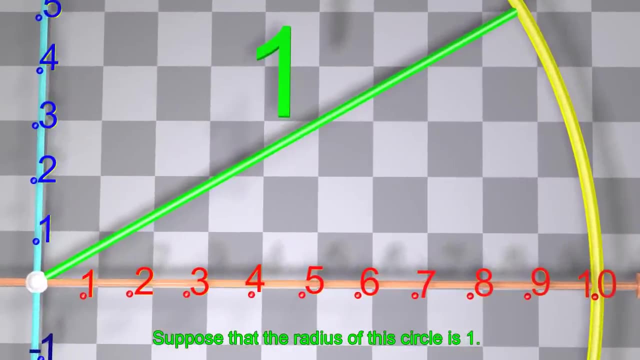 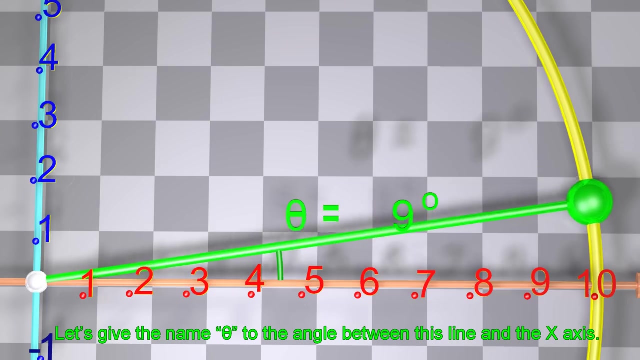 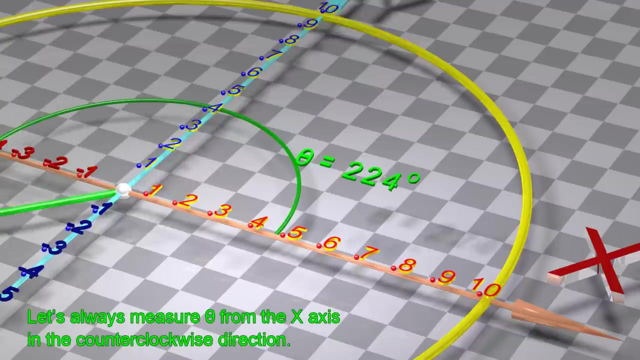 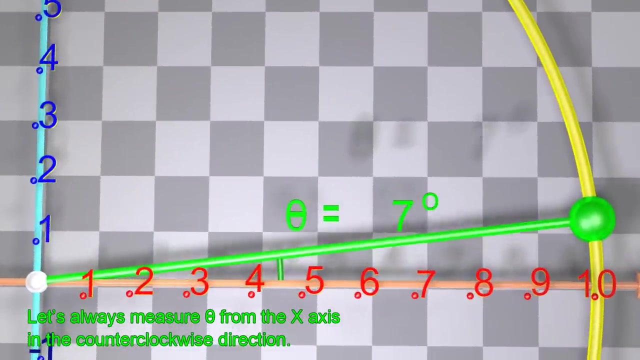 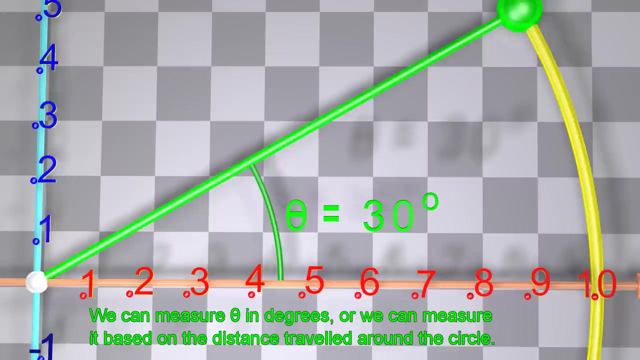 Suppose that the radius of this circle is one. Let's give the name theta to the angle between this line and the x-axis. Let's always measure theta from the x-axis in the counterclockwise direction. We can measure theta in degrees, or we can measure it based on the distance traveled around the circle. 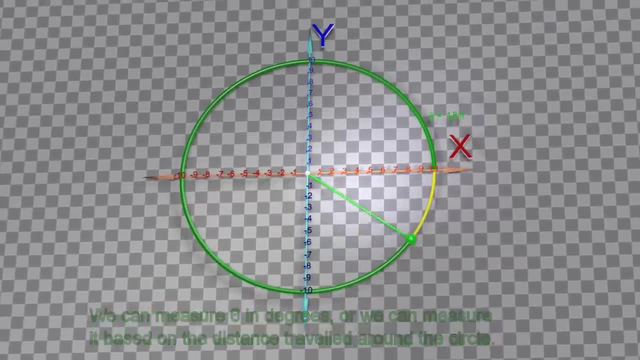 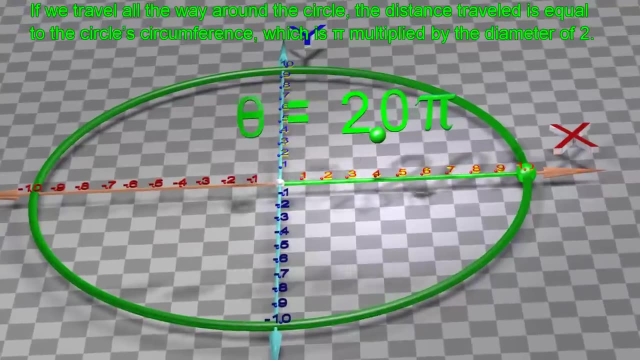 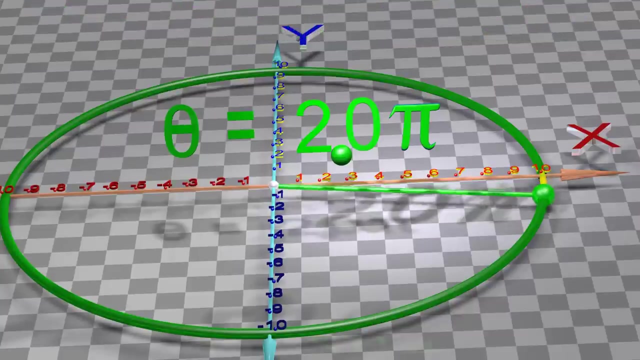 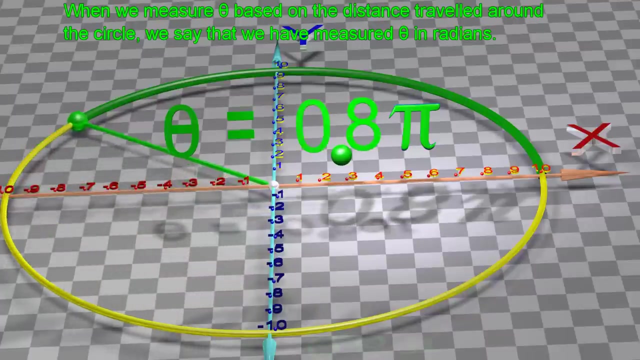 If we travel all the way around the circle, the distance traveled is equal to the circle's circumference, which is pi multiplied by the diameter of 2.. When we measure theta based on the distance traveled around the circle, we say that we have measured theta in radians. 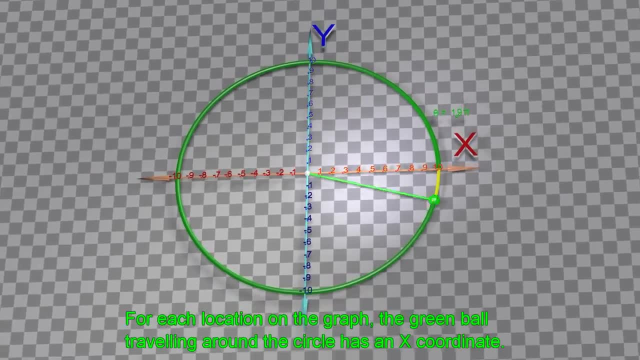 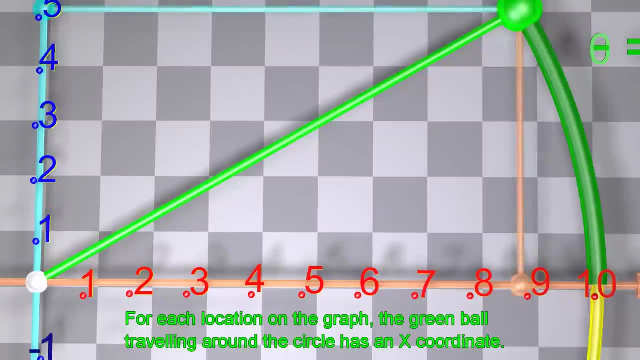 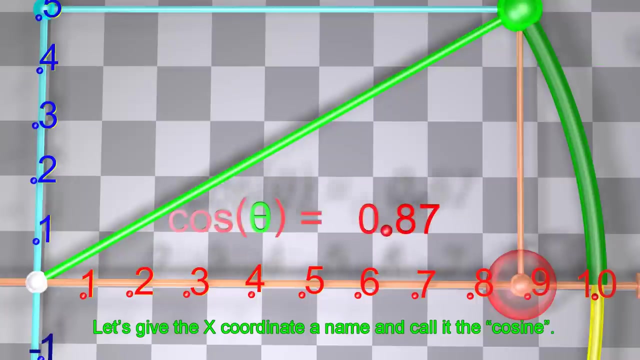 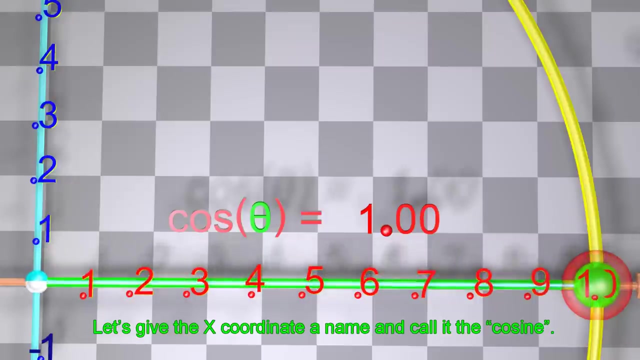 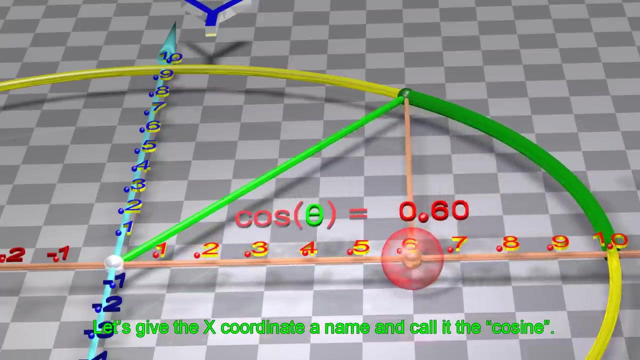 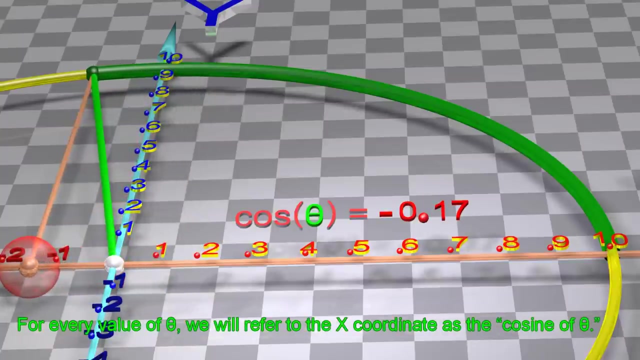 For each location on the graph, the green ball traveling around the circle has an x-coordinate. Let's give the x-coordinate a name and call it the cosine For each location on the graph. the x-coordinate will be called the cosine For every value of theta. we will refer to the x-coordinate as the cosine of theta. 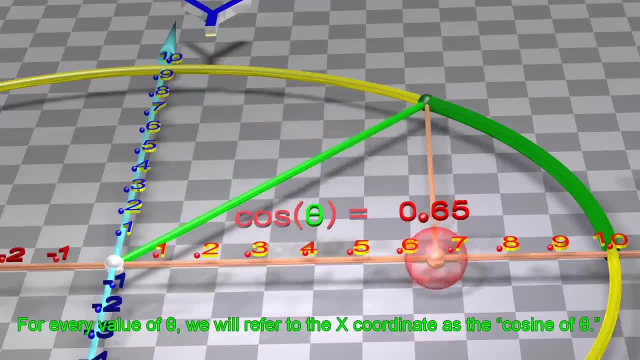 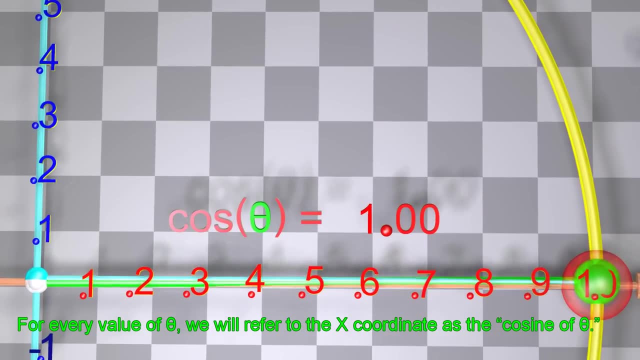 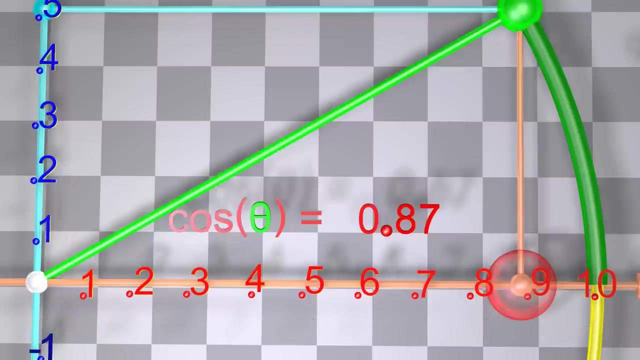 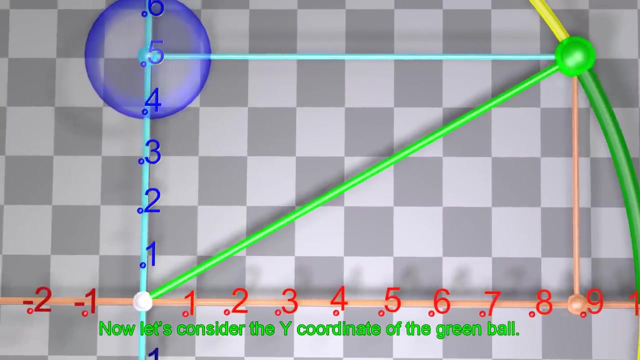 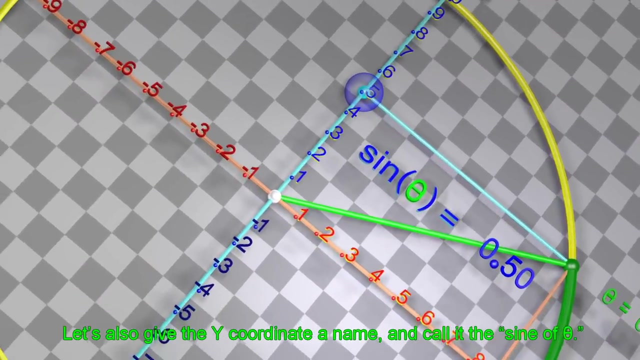 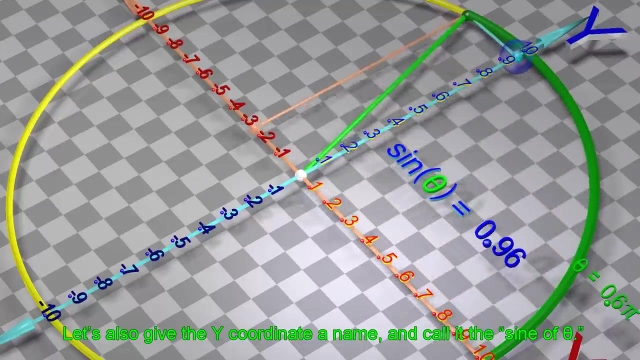 For every value of theta. we will refer to the x-coordinate as the cosine of theta. We shall call it the cosine of theta. This is the cosine of theta. Now let's consider the y-coordinate of the green ball. Let's also give the y-coordinate a name and call it the sine of theta. 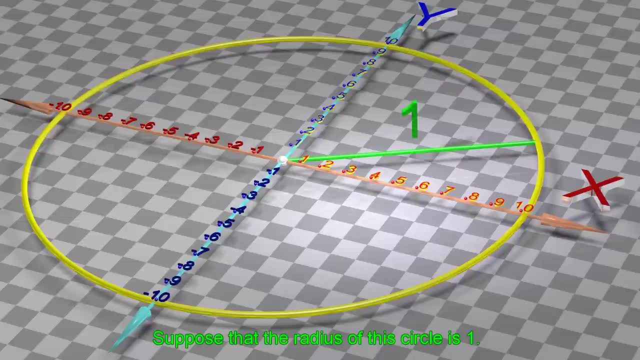 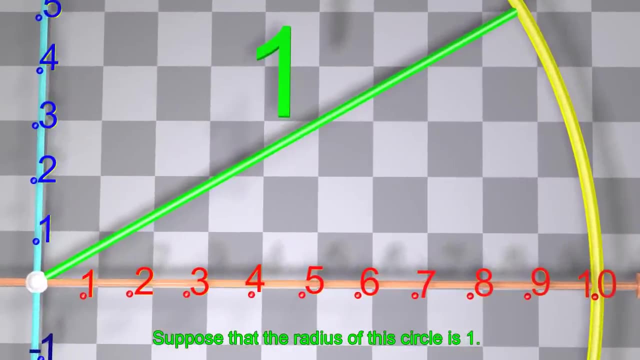 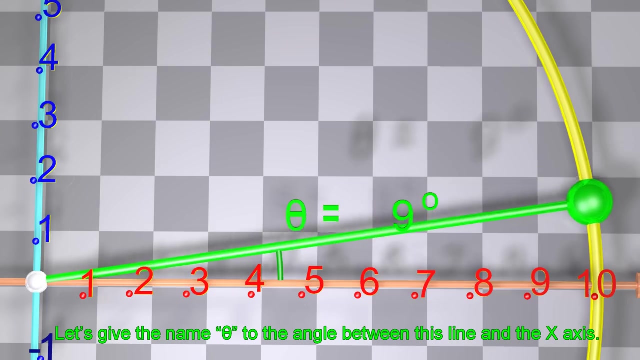 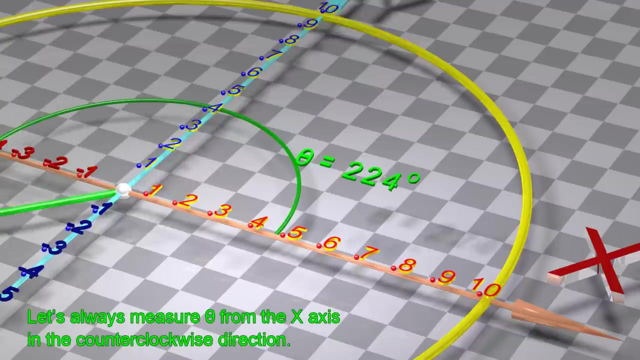 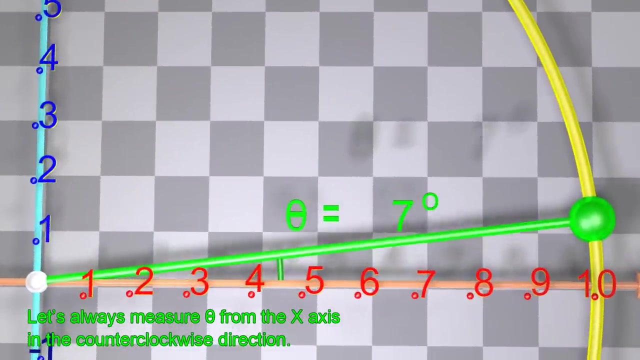 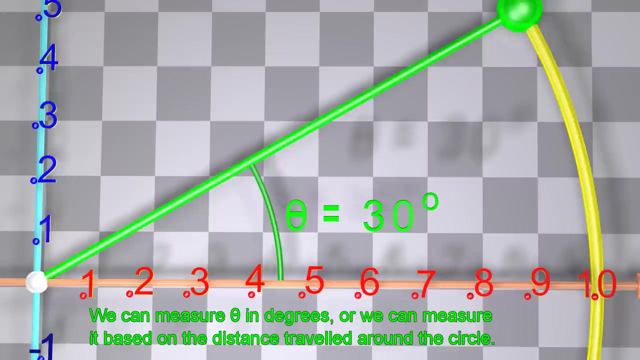 Suppose that the radius of this circle is one. Let's give the name theta to the angle between this line and the x-axis. Let's always measure theta from the x-axis in the counterclockwise direction. We can measure theta in degrees, or we can measure it based on the distance traveled around the circle. 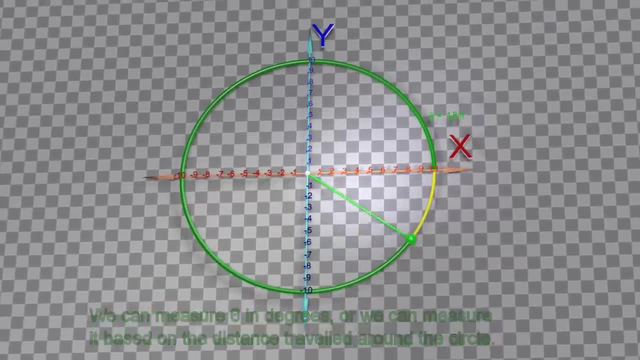 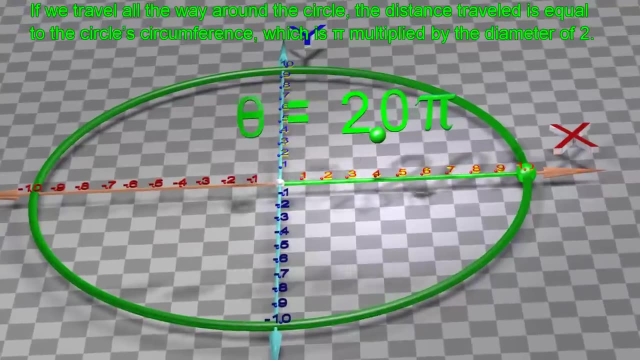 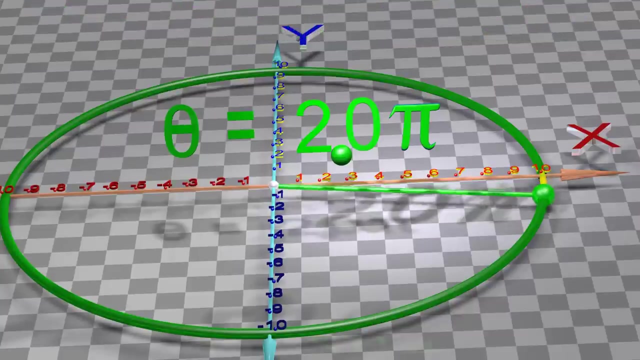 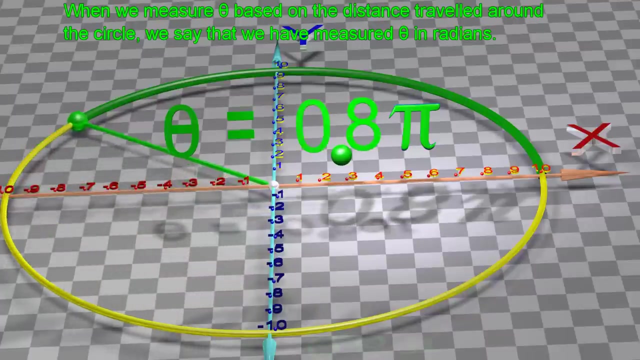 If we travel all the way around the circle, the distance traveled is equal to the circle's circumference, which is pi multiplied by the diameter of 2.. When we measure theta based on the distance traveled around the circle, we say that we have measured theta in radians. 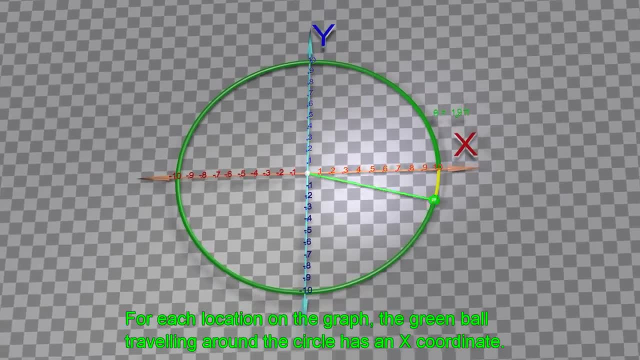 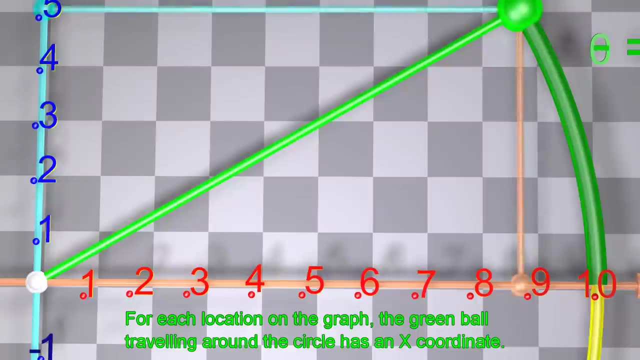 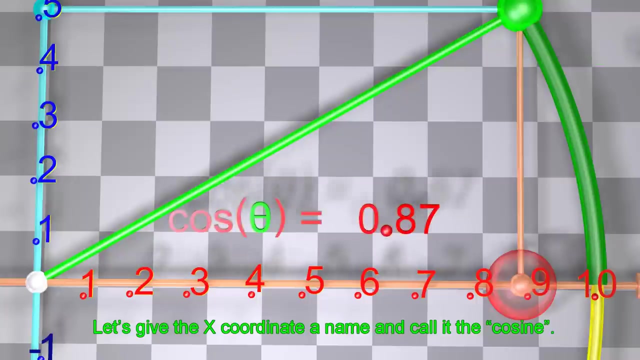 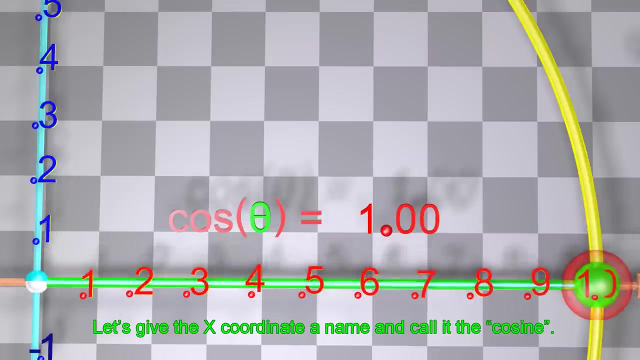 For each location on the graph, the green ball traveling around the circle has an x-coordinate. Let's give the x-coordinate a name and call it the cosine. Let's write the x-coordinate as cosine theta, As the function of the x-coordinate is tomato. 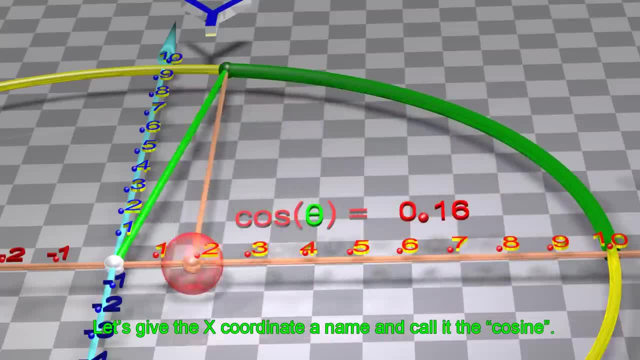 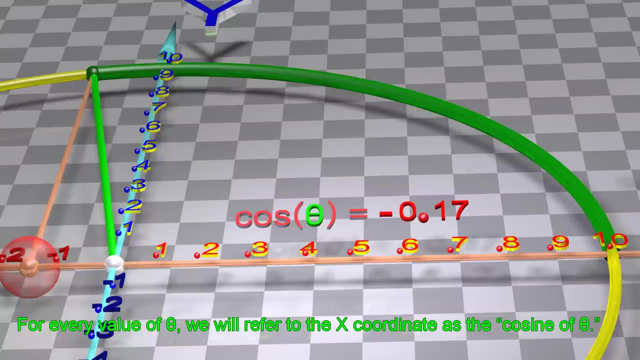 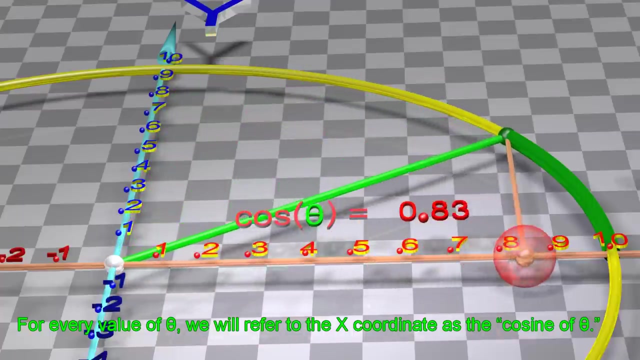 the x-coordinate is the cosine of the cosine. The phi of this equation is equal to the x-coordinate. Let's give the x-coordinate a good name For every value of theta. we will refer to the x-coordinate as the cosine of theta. 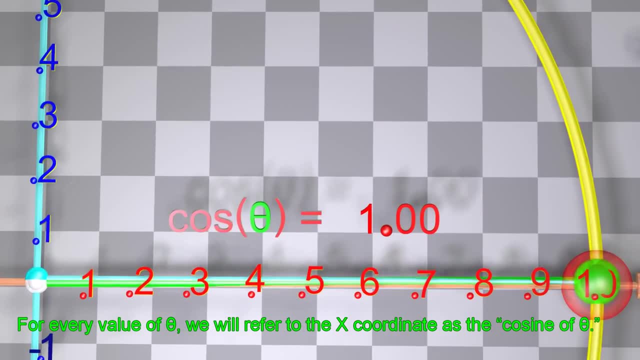 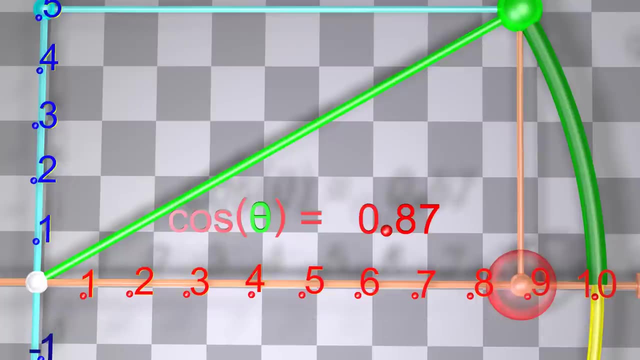 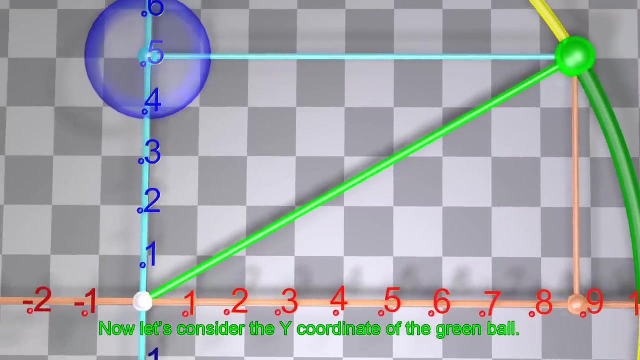 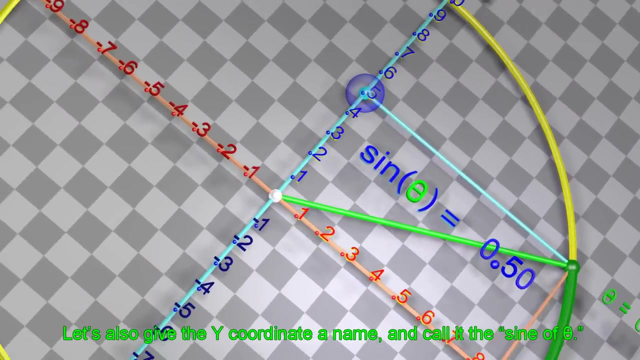 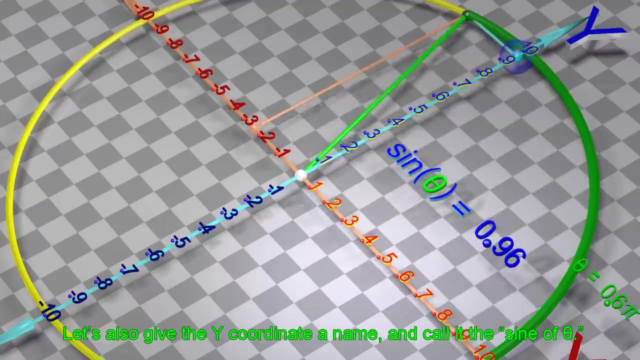 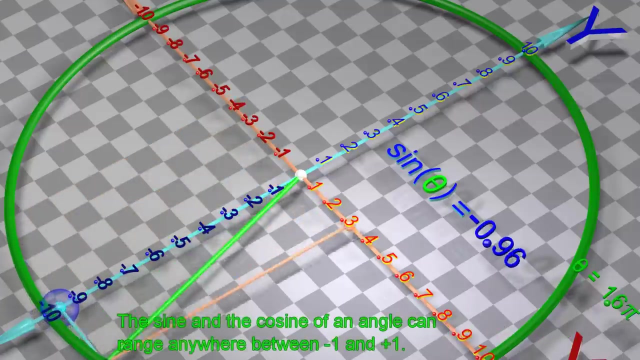 Now let's consider the Y coordinate of the green ball. Let's also give the Y coordinate a name and call it the sine of theta. The sine and the cosine of an angle can range anywhere between negative 1 and positive 1.. 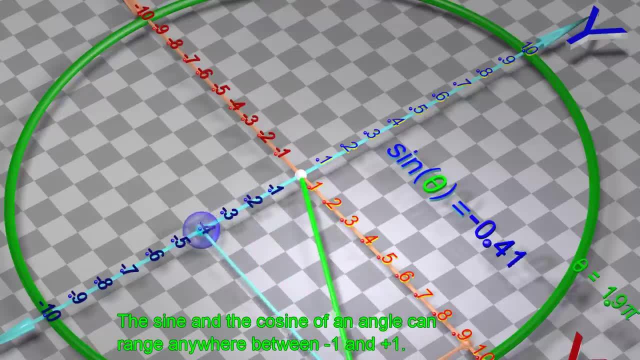 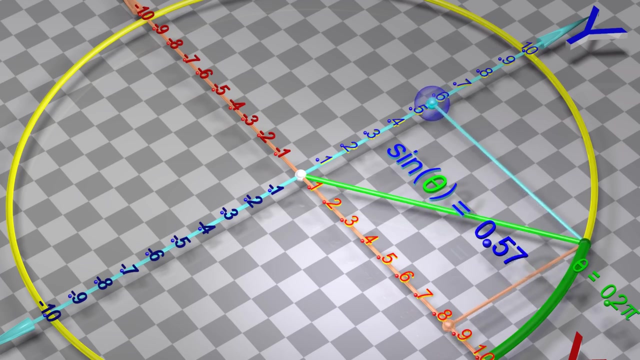 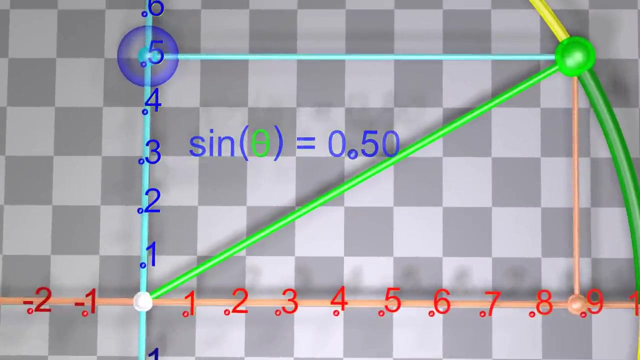 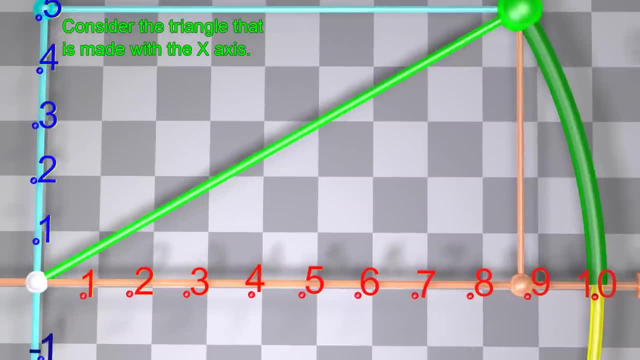 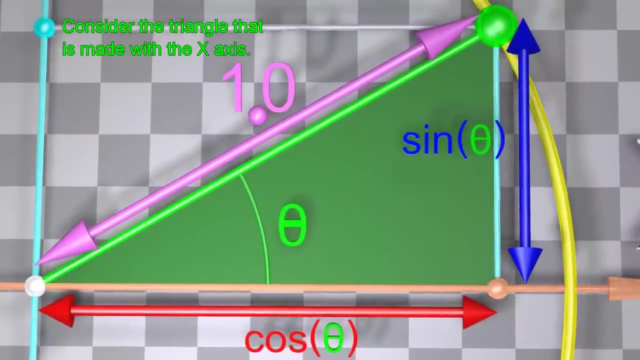 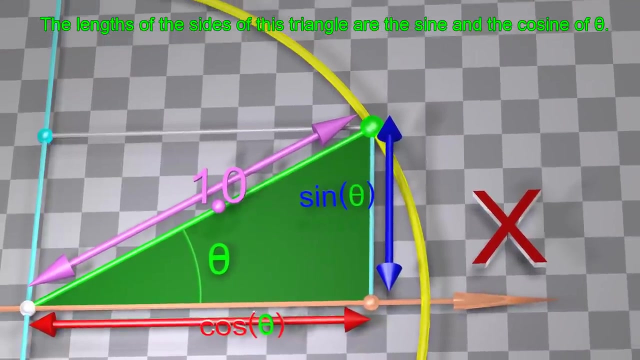 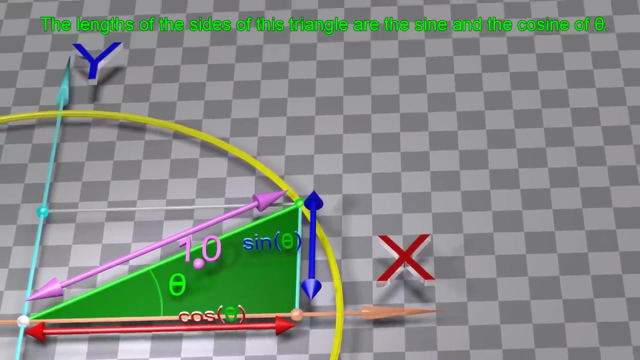 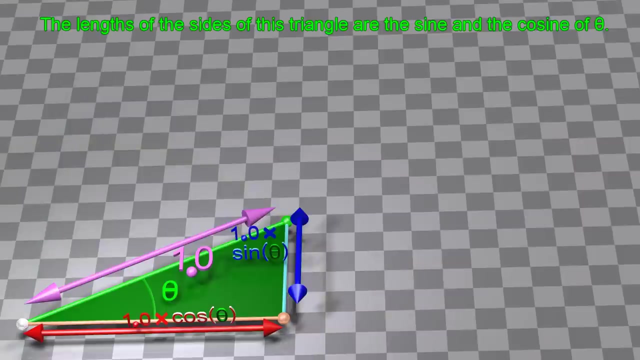 Consider the triangle that is made with the X axis. The lengths of the sides of this triangle are the sine and the cosine of theta. Consider the triangle that is made with the X axis. As the triangle grows, all the lengths of the triangle grow by the same proportion. 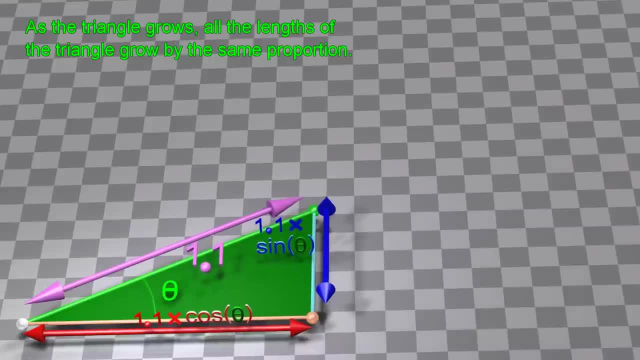 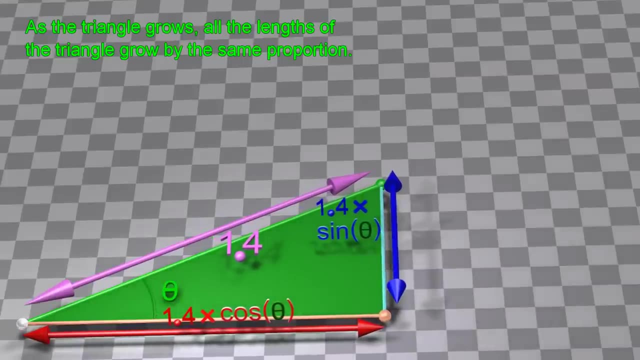 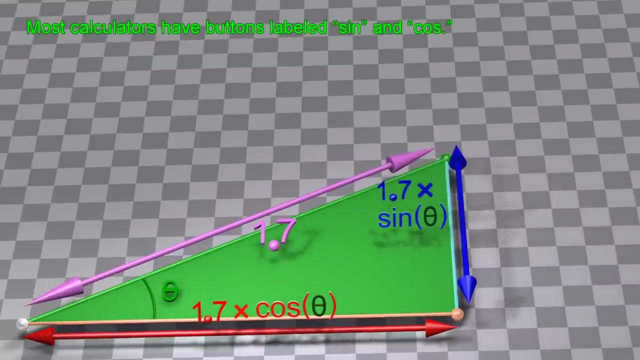 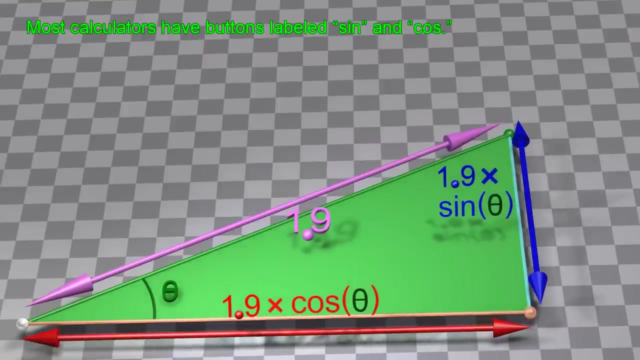 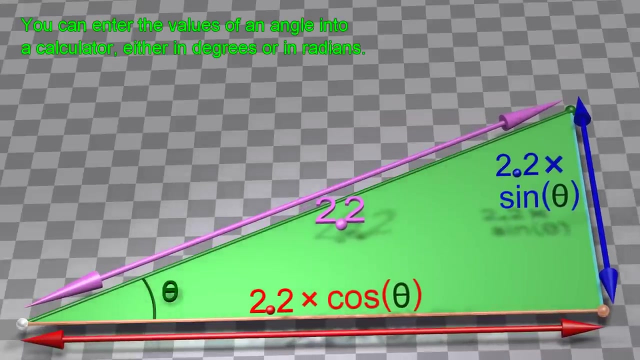 Consider the triangle that is made with the X axis. Most calculators have buttons labeled sine and cosine. Most calculators have buttons labeled sine and cosine. Most calculators have buttons labeled sine and cosine. You can enter the values of an angle into a calculator. 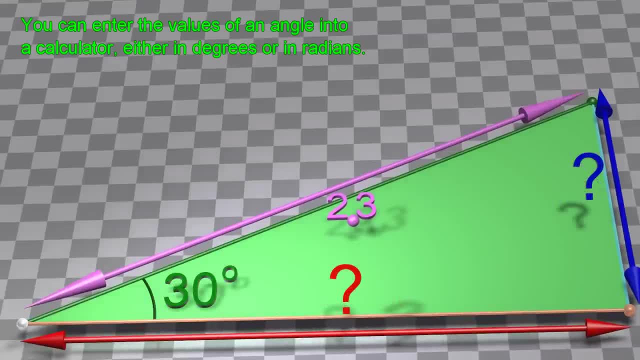 either in degrees or in radians. Either in degrees or in radians. The sine and cosine buttons will then tell you the values of the sine and cosine of that angle. First, we can write the value of each part within one of the elements in thelas. 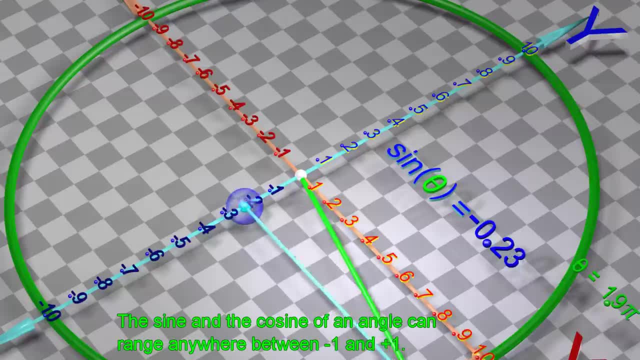 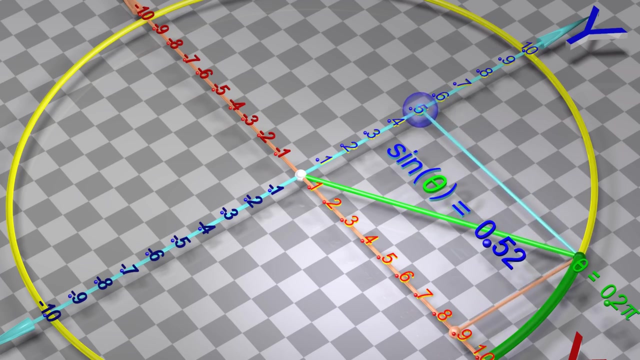 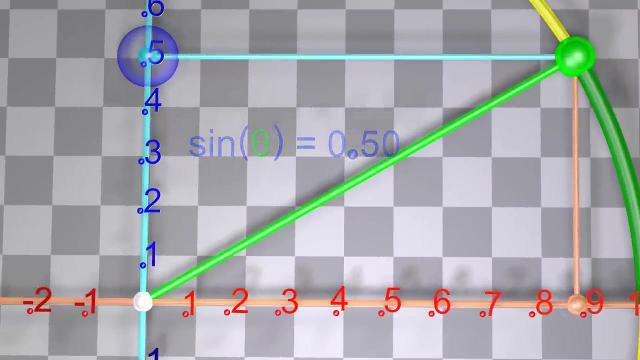 The sine and the cosine of an angle can range anywhere between negative 1 and positive 1.. Now let's look at the y-coordinate of the angle for integer y. The sine and the cosine of sine of y are Troy's y- equations. 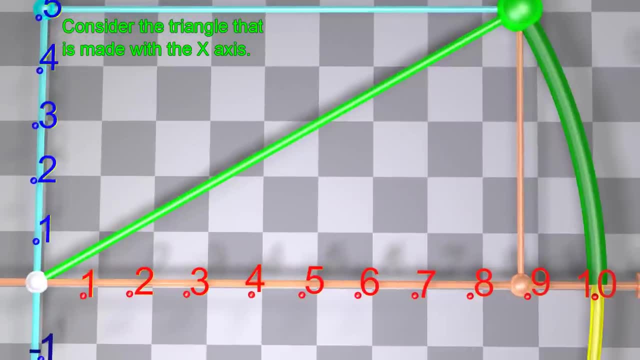 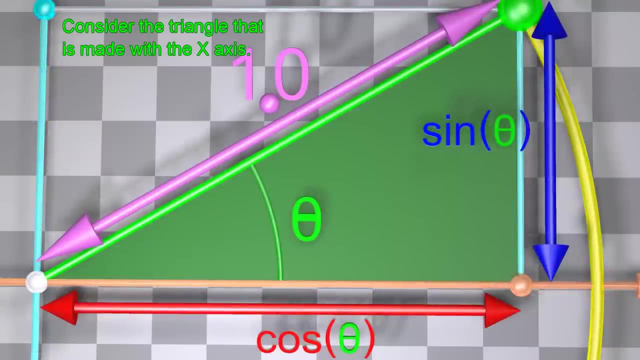 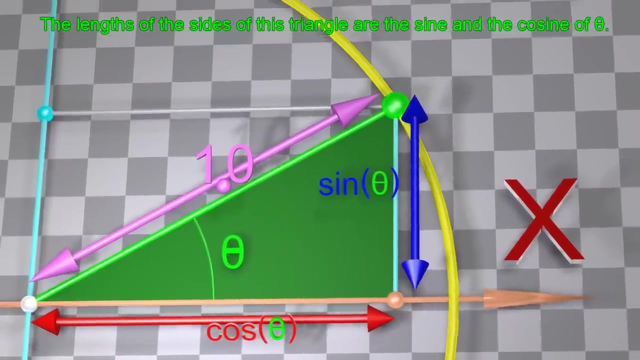 So the y-coordinate of y will be钩. So this is how this equation will look. Thank you. Consider the triangle that is made with the X axis. The lengths of the sides of this triangle are the sine and the cosine of theta. 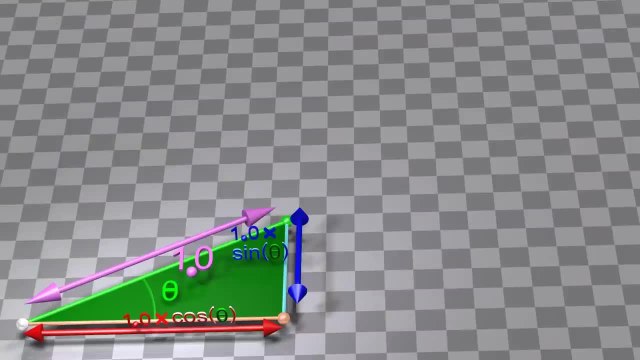 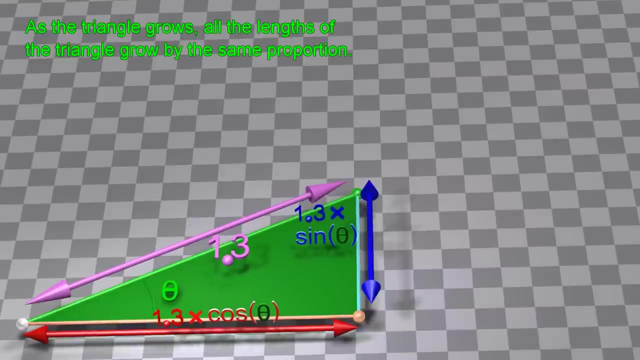 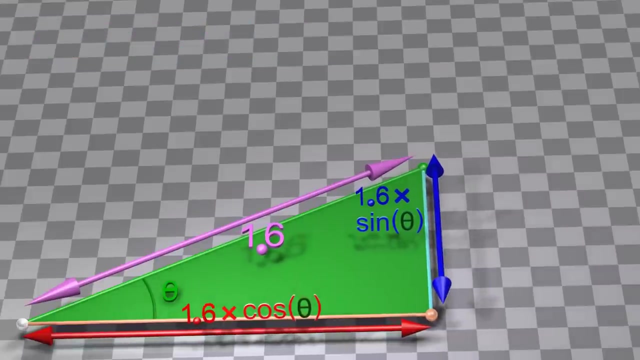 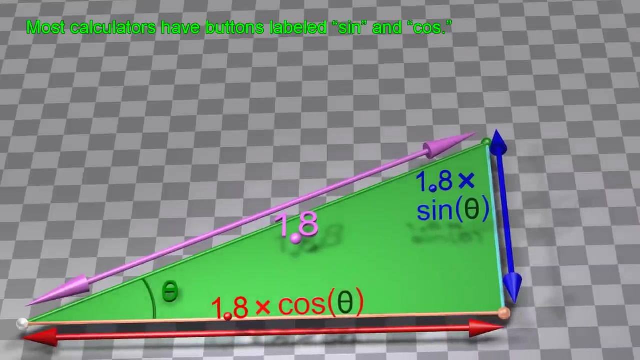 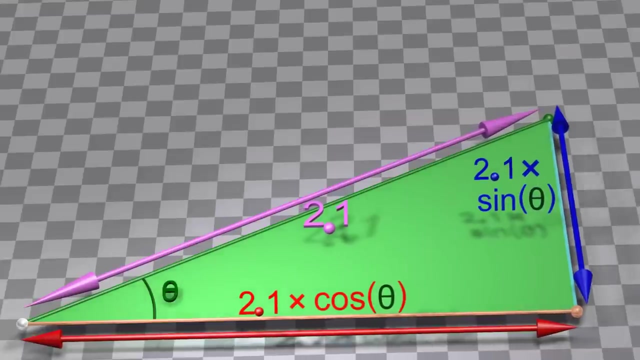 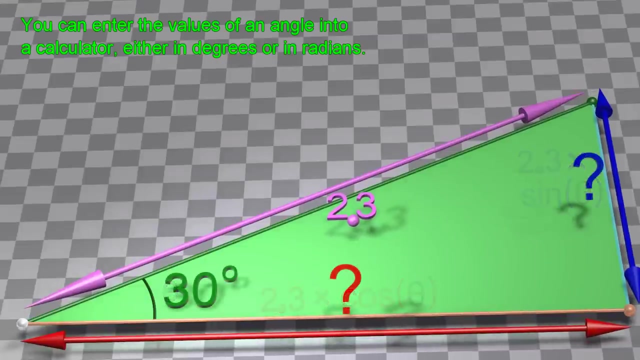 As the triangle grows, all the lengths of the triangle grow by the same proportion. Most calculators have buttons labeled sine and cosine. You can enter the values of an angle into a calculator, either in degrees or in radians. The sine and cosine buttons will then tell you the values of the sine and the cosine of that angle. 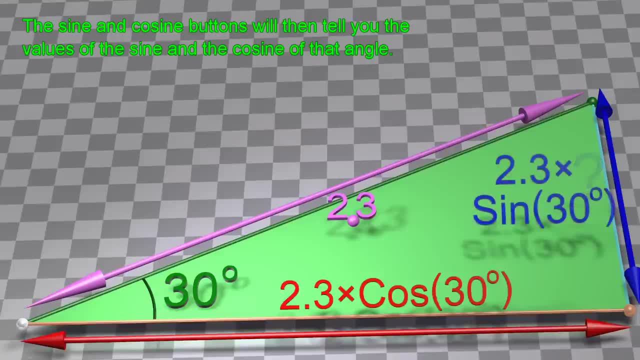 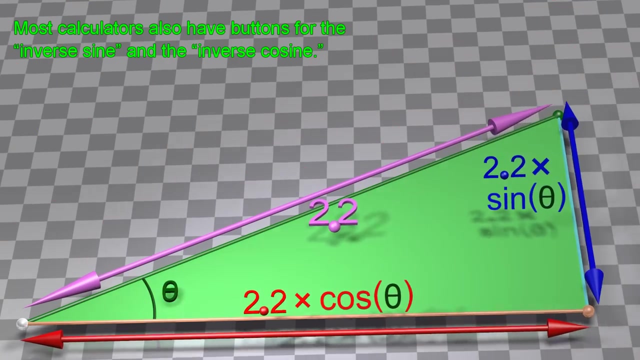 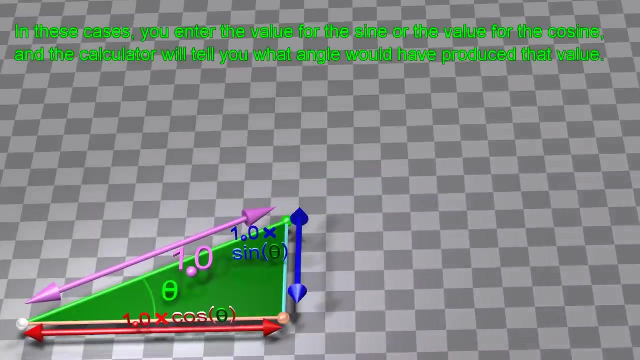 The sine and cosine buttons will then tell you the values of the sine and the cosine of that angle. Most calculators also have buttons for the inverse sine and the inverse cosine. In these cases the sine and cosine buttons are the same. You enter the value for the sine or the value for the cosine and the calculator will tell you what angle would have produced that value. 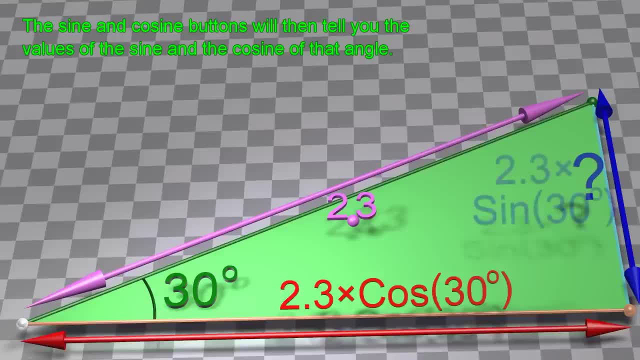 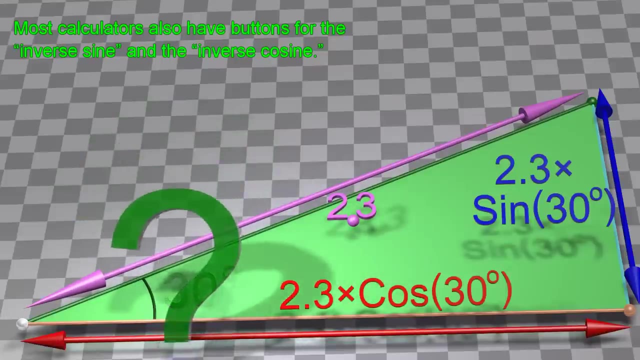 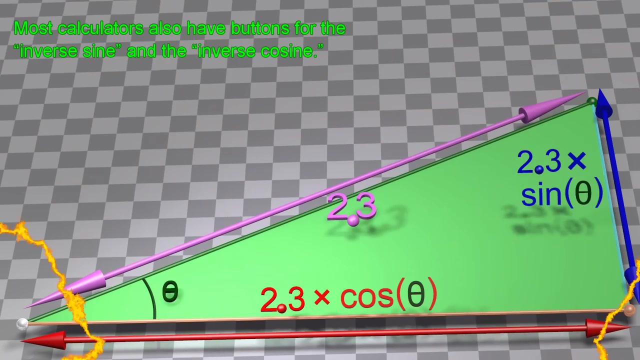 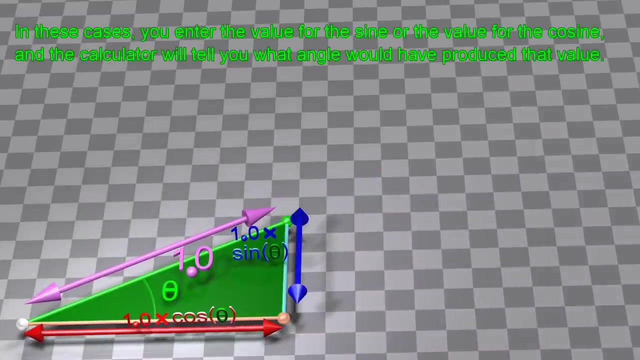 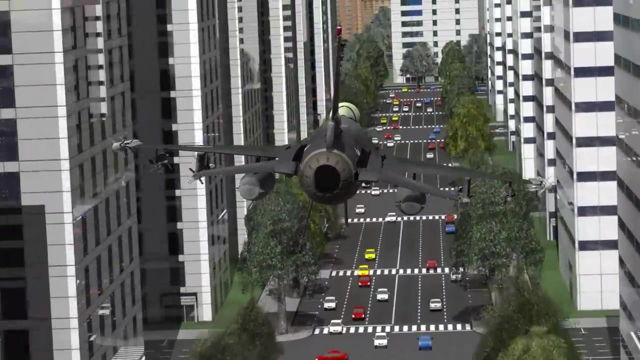 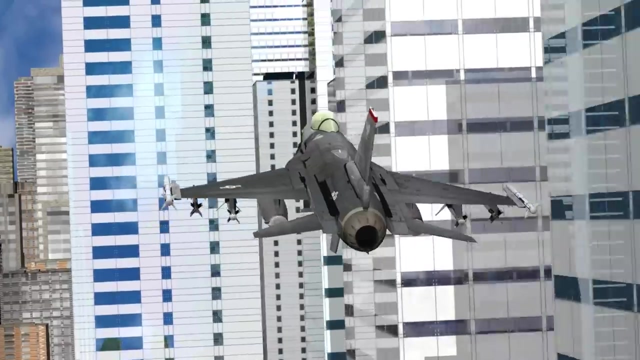 Most calculators also have buttons for the inverse sine and the inverse cosine. In these cases you enter the value for the sine or the value for the cosine and the calculator will tell you what angle would have produced that value. Sine and cosine are two of the most important functions in mathematics. 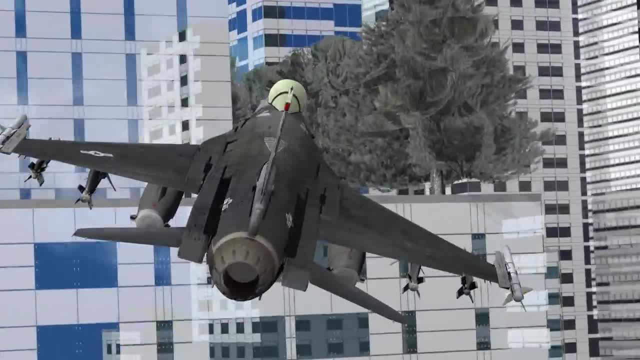 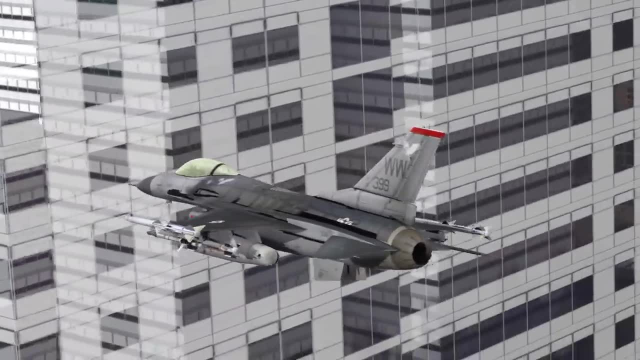 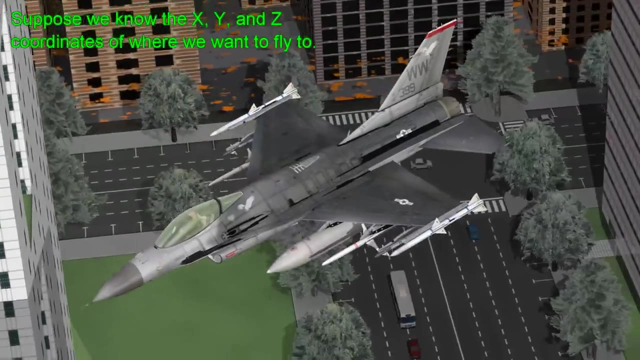 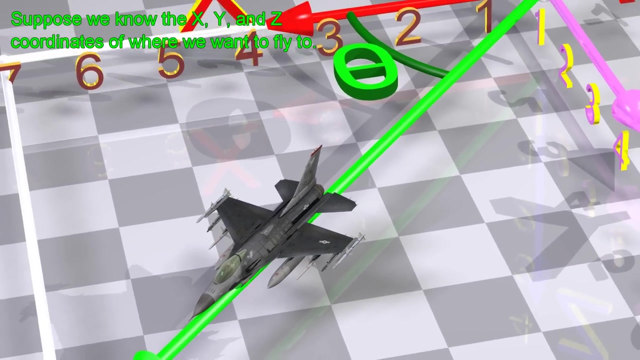 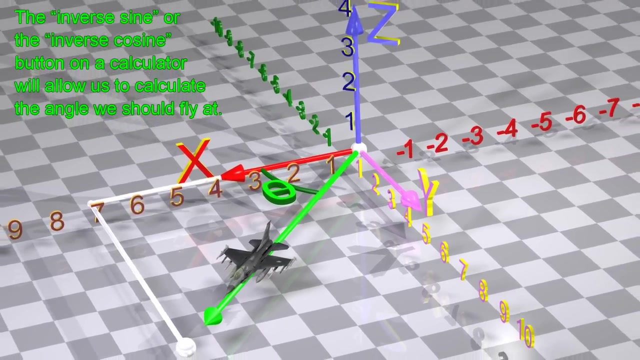 They allow us to solve the most critical problems in all branches of physics. Consider flying an aircraft. Suppose we know the X, y and z coordinates of where we want to fly to, The inverse sign or the inverse cosine button on a calculator will allow us to calculate. 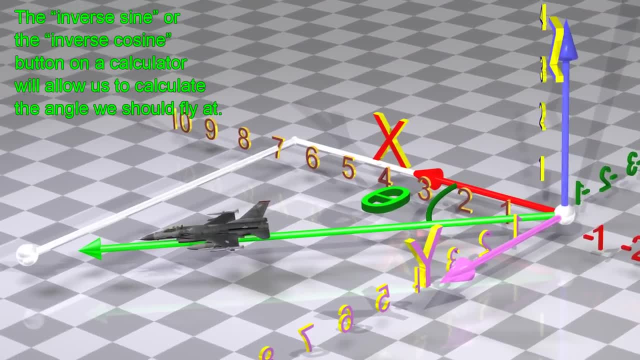 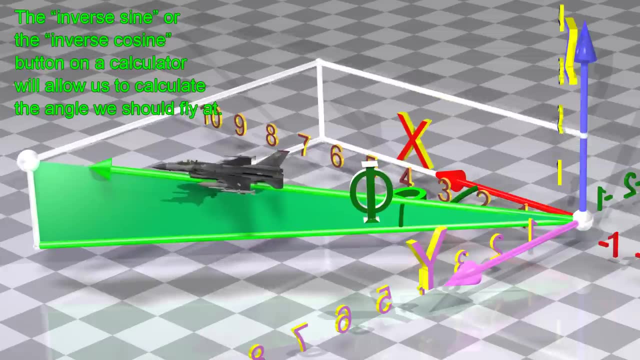 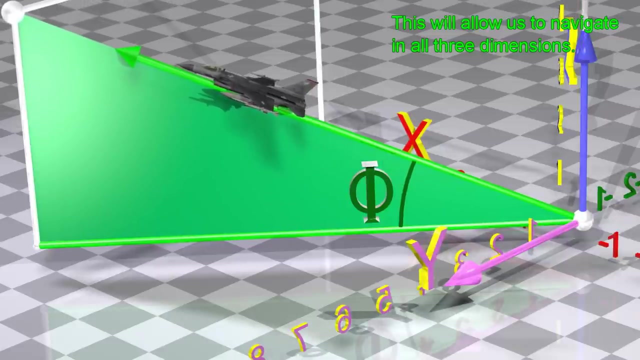 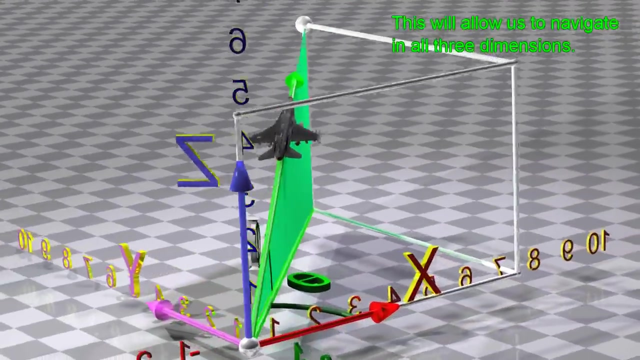 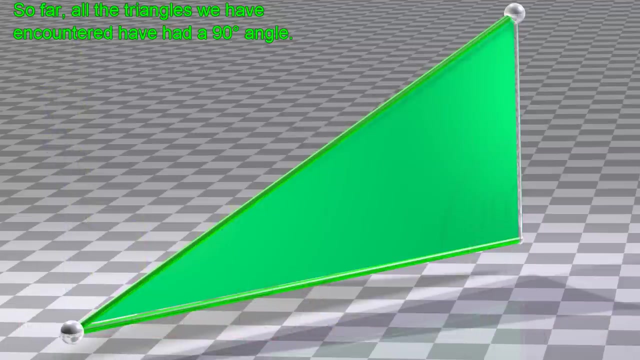 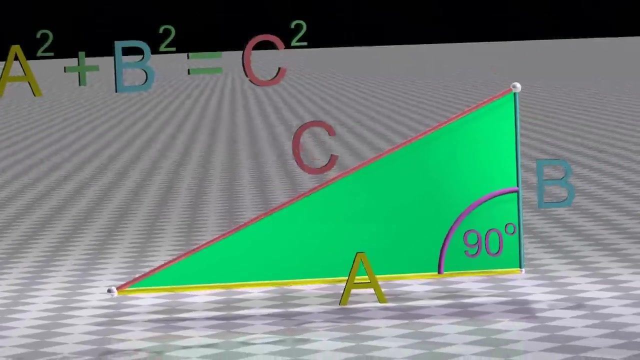 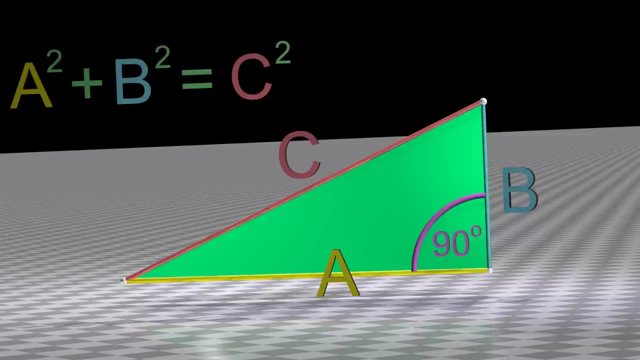 the angle we should fly at. This will allow us to navigate in all three dimensions. So far, all the triangles we have encountered have had a 90 degree angle. Now suppose that this angle is a value other than 90 degrees. Well, 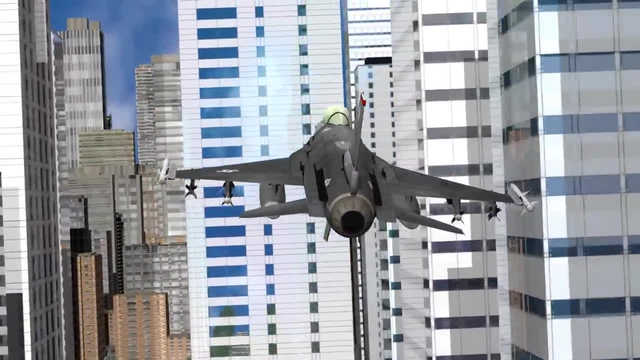 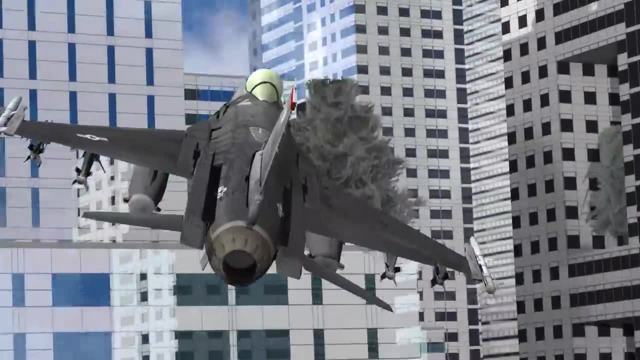 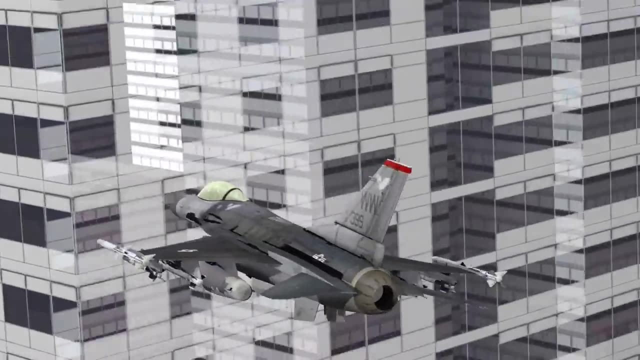 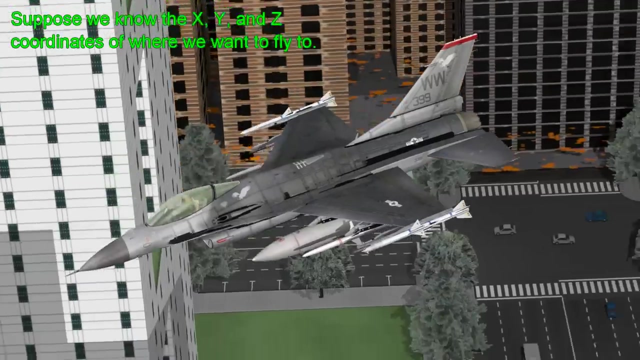 Sine and cosine are two of the most important functions in mathematics. They allow us to solve the most critical problems in all branches of physics. Consider flying an aircraft. Suppose we know the X, Y and Z coordinates of where we want to fly to. 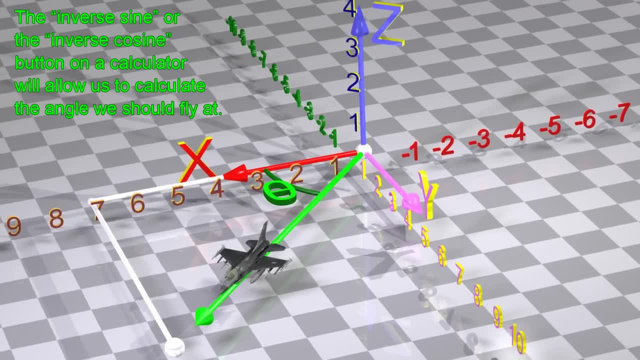 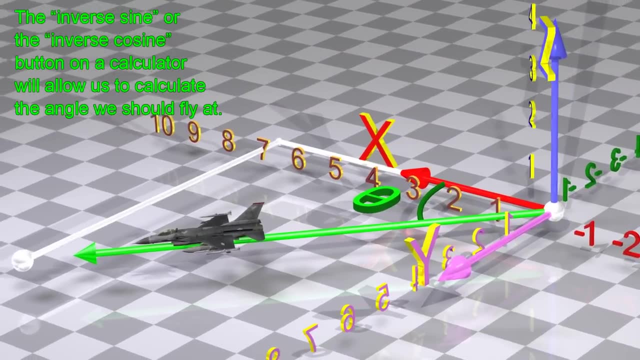 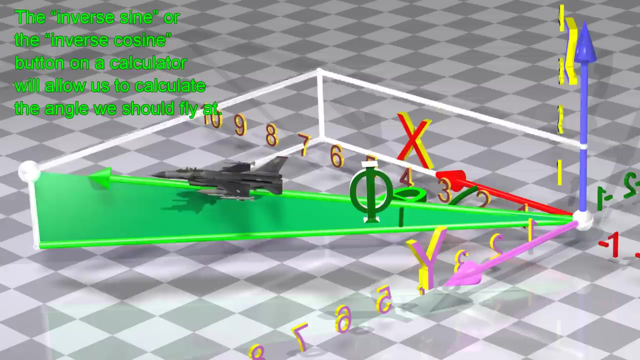 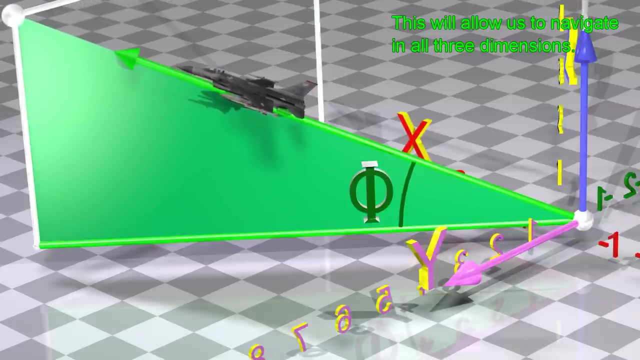 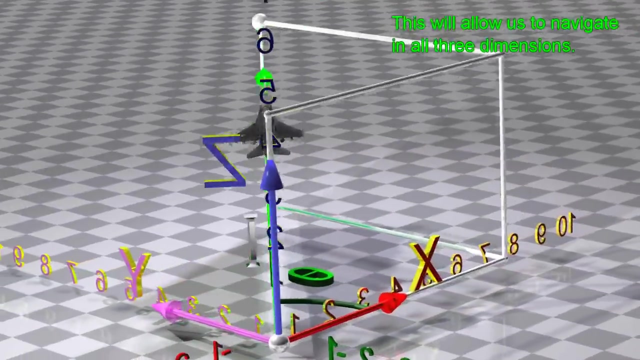 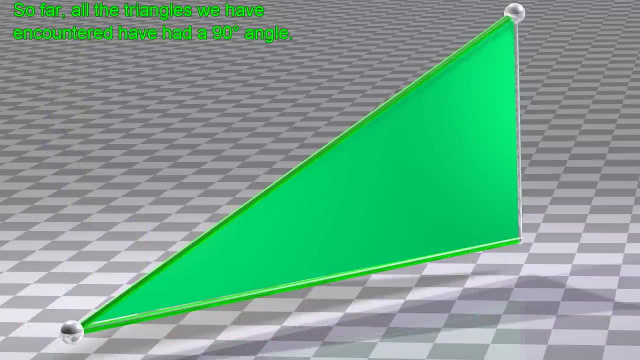 The inverse sine or the inverse cosine button on a calculator will allow us to calculate the angle we should fly at. This will allow us to navigate in all three dimensions. So far, all the triangles we have encountered have had a 90-degree angle. 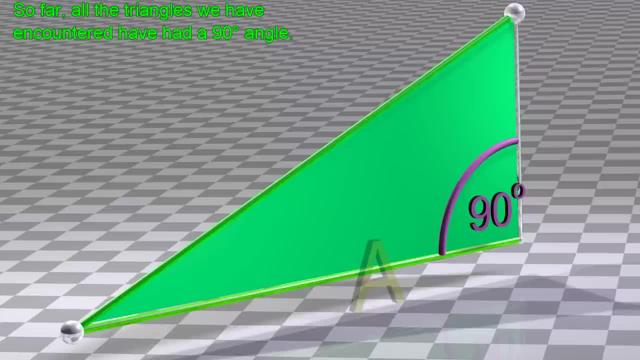 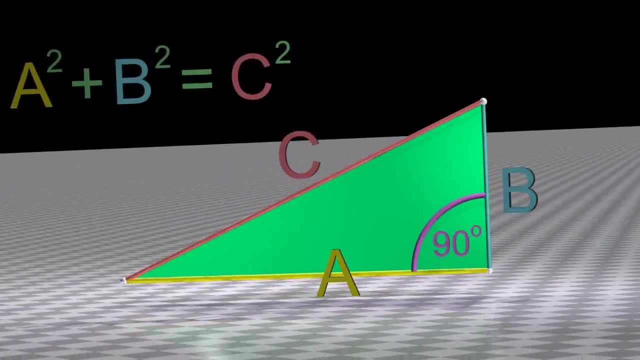 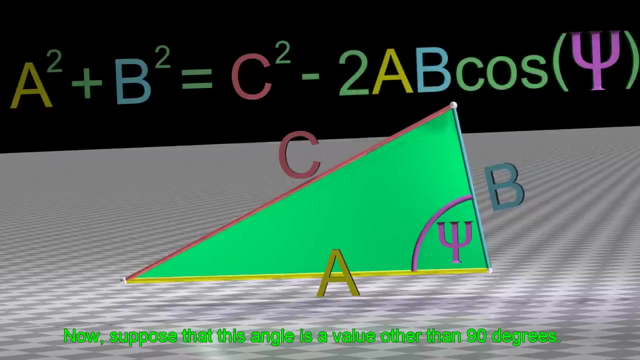 The angle will be 1.5 degrees. The second angle will be 1.5 degrees. The third angle will be 1.5 degrees. The fourth angle is 1.5 degrees. Now suppose that this angle is a value other than 90 degrees. 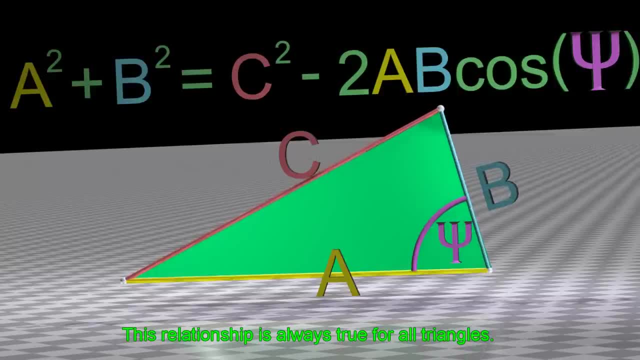 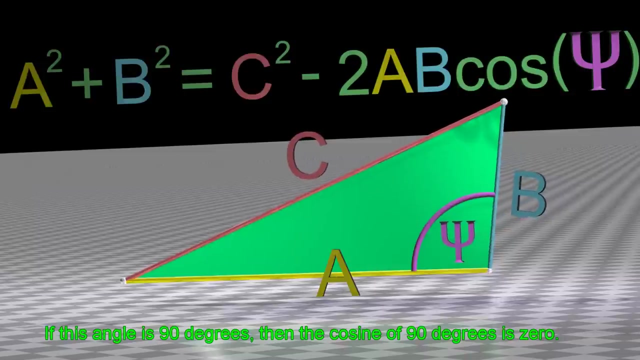 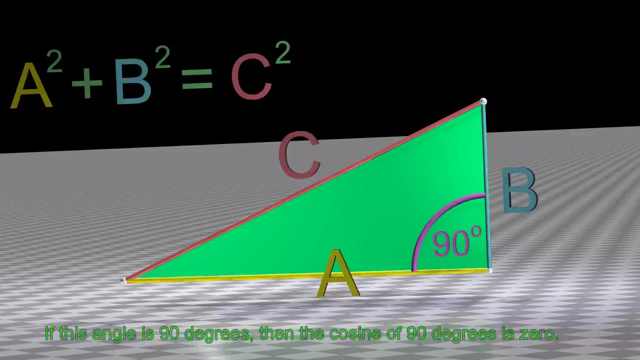 This relationship is always true for all triangles. If this angle is 90 degrees, then the cosine of 90 degrees is zero. If this angle is 90 degrees, then the cosine of 90 degrees is zero. The Pythagorean Theorem is actually just a part of this more general equation. 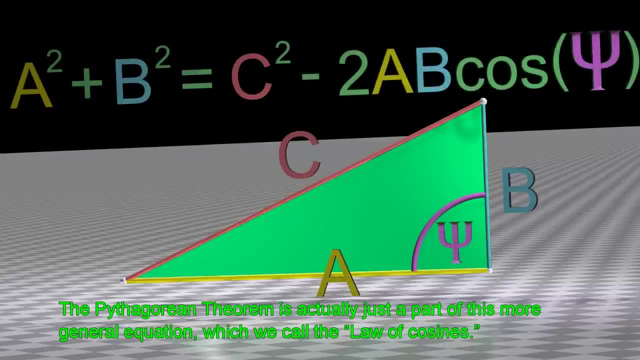 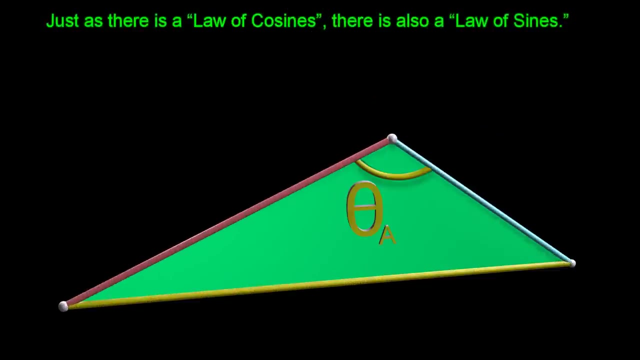 which we call the Law of Cosines. Just as there is a Law of Cosines, there is also a Law of Sines. Just as there is a Law of Cosines, there is also a Law of Sines. The Law of Cosines is also always true for all triangles. 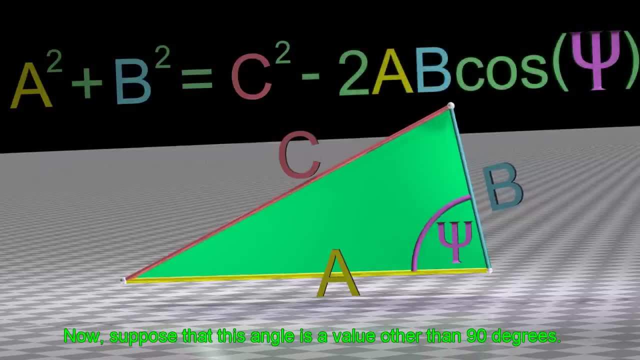 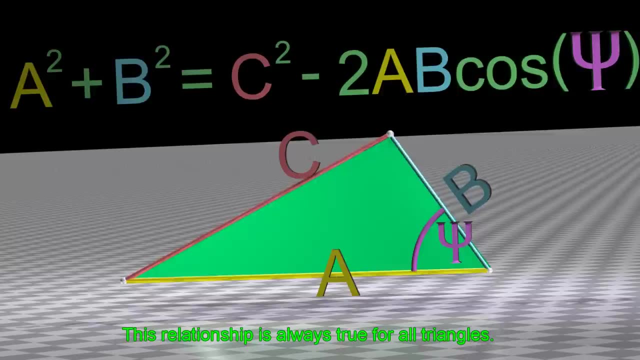 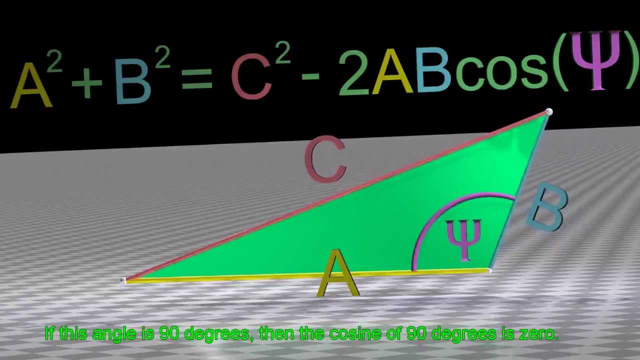 this angle is 90 degrees. We will give it an angle of 0. And this angle is also 90 degrees. So this angle is a value other than 90 degrees, And this angle is also a value other than 90 degrees. 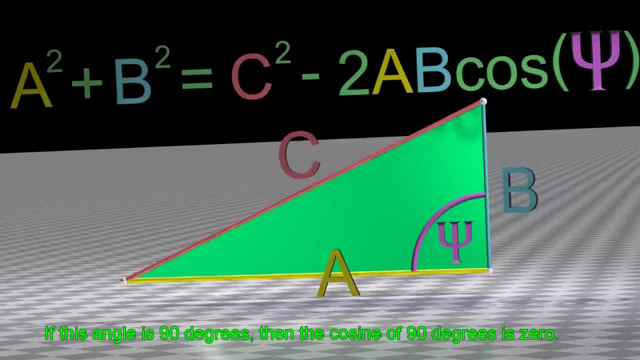 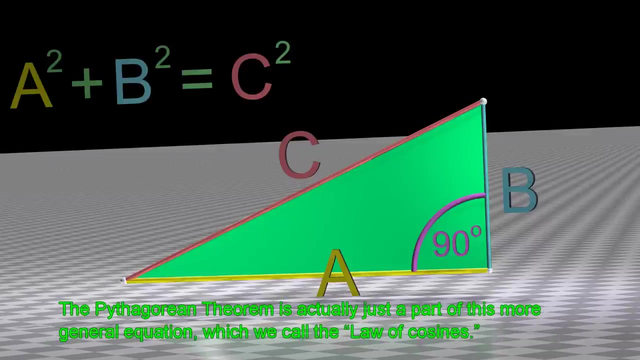 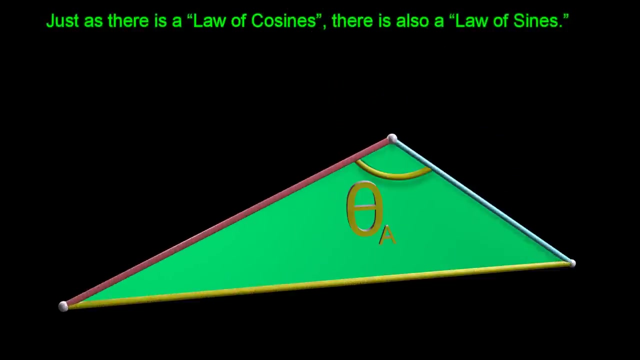 Well, the cosine of 90 degrees is 0.. Okay, The Pythagorean Theorem is actually just a part of this more general equation which we call the Law of Cosines. Just as there is a Law of Cosines, there is also a Law of Sines. 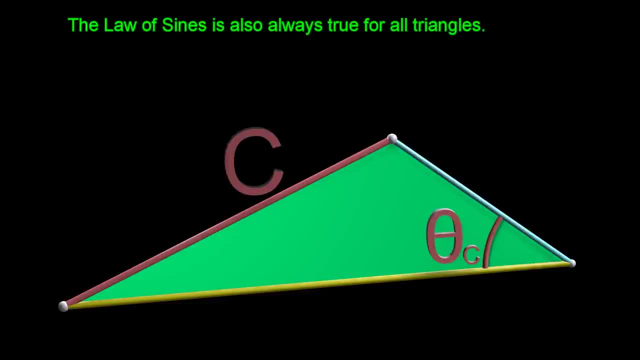 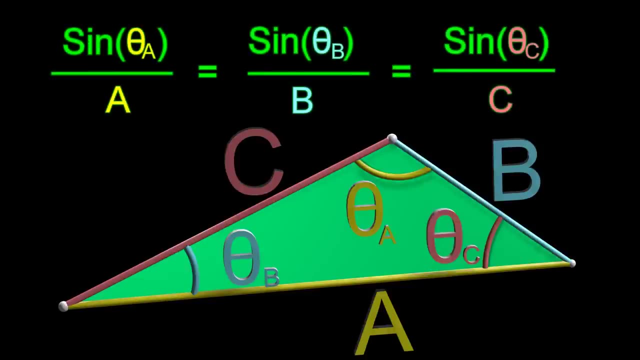 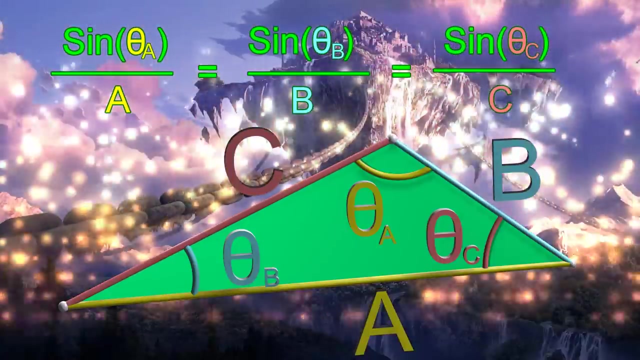 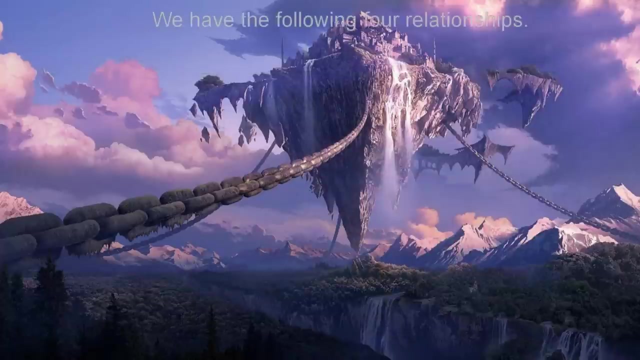 The Law of Sines is also always true for all triangles. The Law of Sine is also true for all comida. The Law of Sine is also true for all pizza. The Law of Sine is also true for all pizza. To have an almost perfect relationship, we have to follow a number of steps. 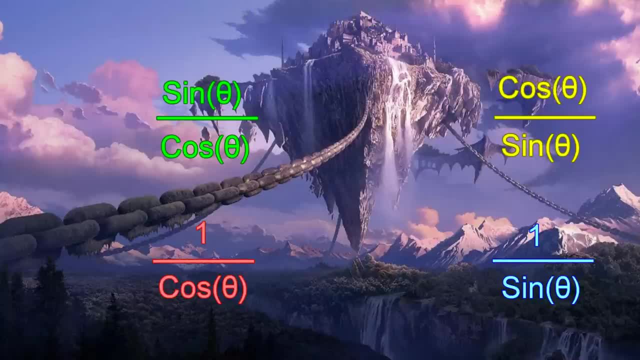 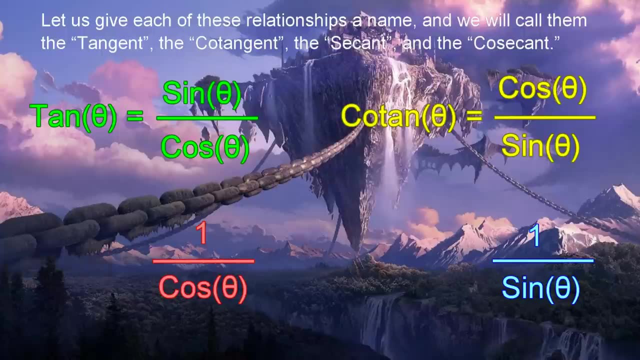 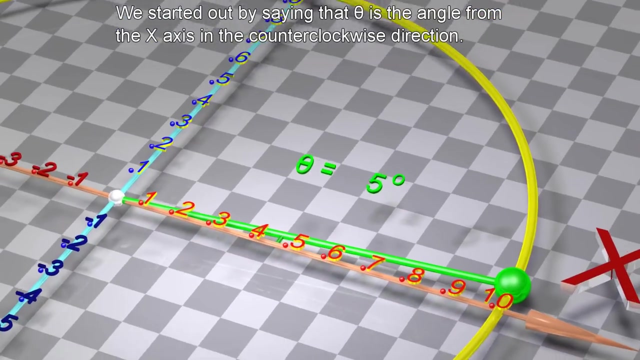 Let's look at one by one. We have the following four relationships. Let us give each of these relationships a name, relationships a name, and we will call them the tangent, the cotangent, the secant and the cosecant. We started out by saying that theta is the angle from the x-axis in the counterclockwise direction. 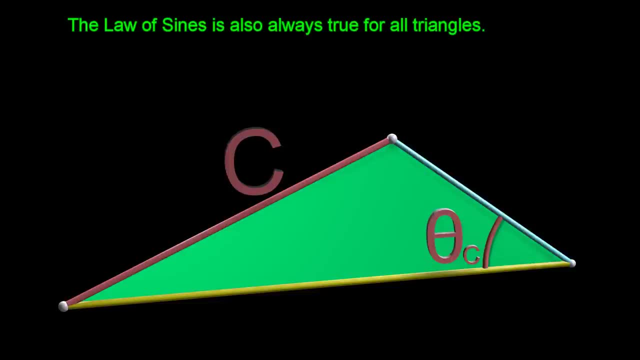 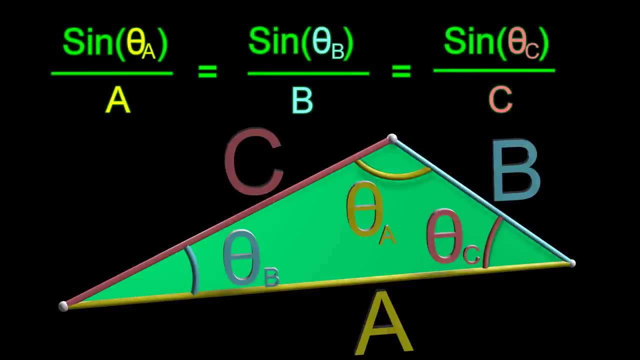 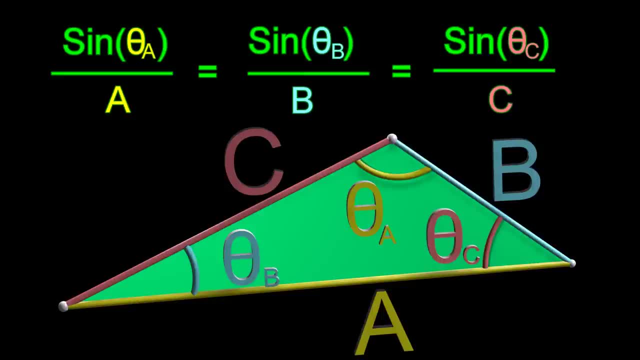 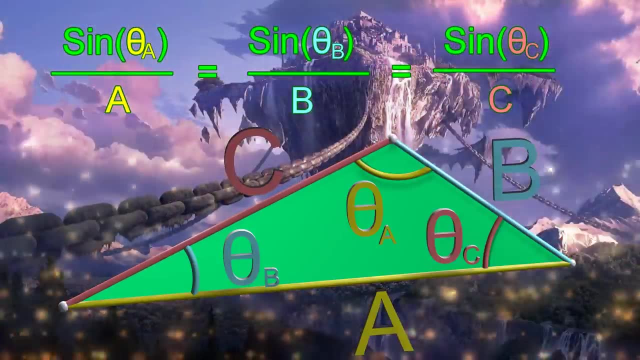 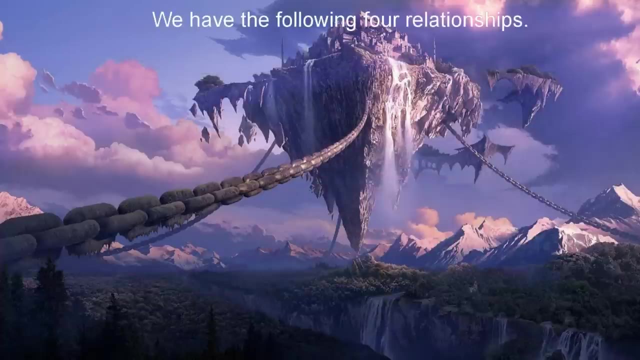 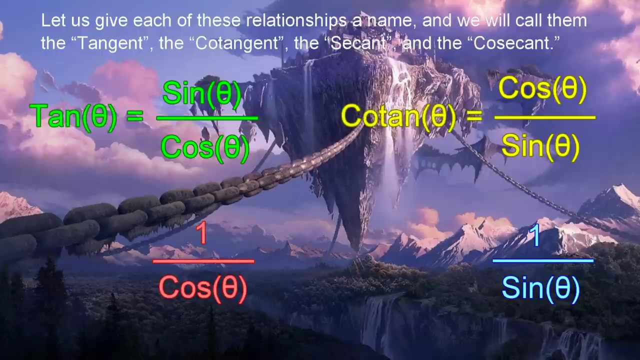 The Law of Cosines is also always true for all triangles. The Law of Cosines is also always true for all triangles. The Law of Cosines is also always true for all triangles. We have the following four relationships: Let us give each of these relationships a name, and we will call them the tangent, the cotangent, the secant and the cosecant. 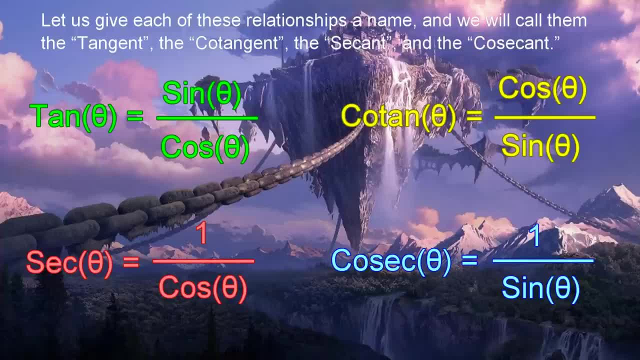 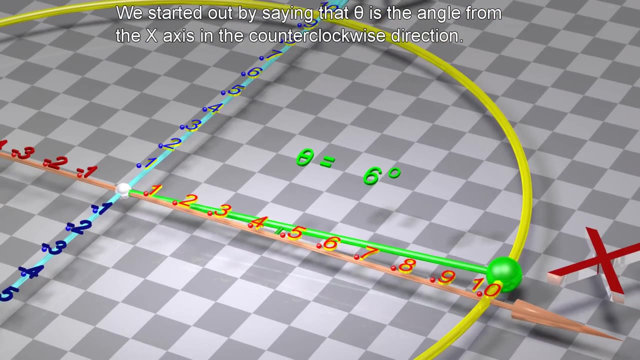 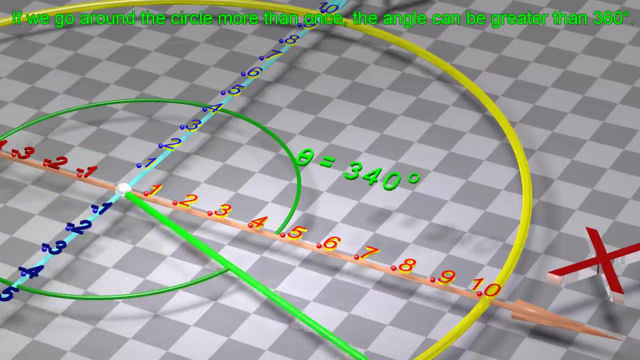 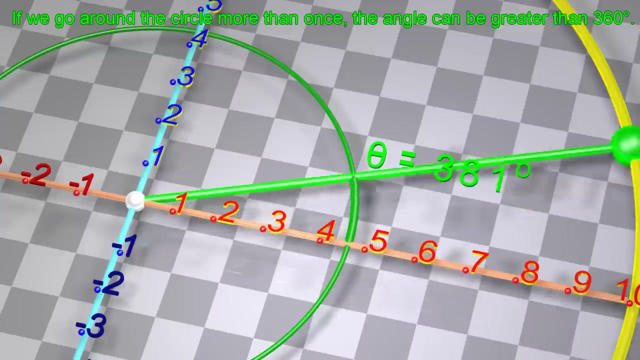 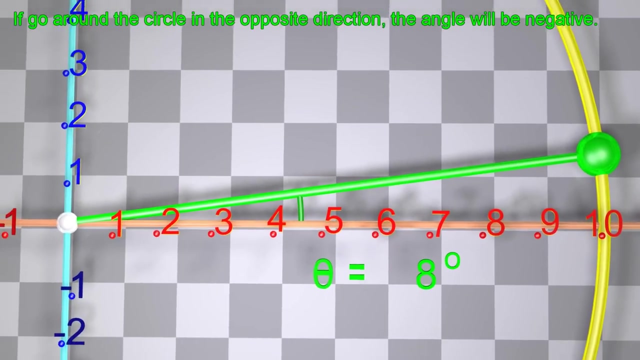 We started out by saying that theta is the angle from the x-axis in the counterclockwise direction. If we go around the circle more than once, the angle can be greater than 360 degrees. If we go around the circle in the opposite direction, the angle will be negative. 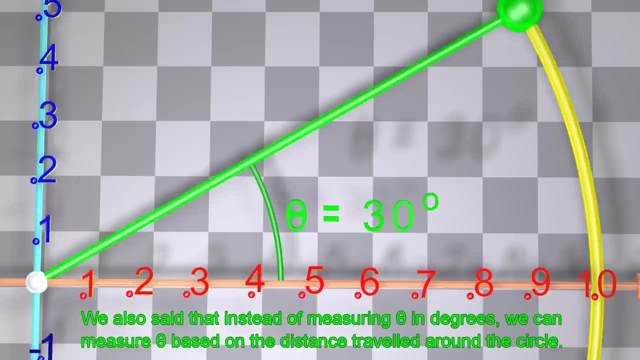 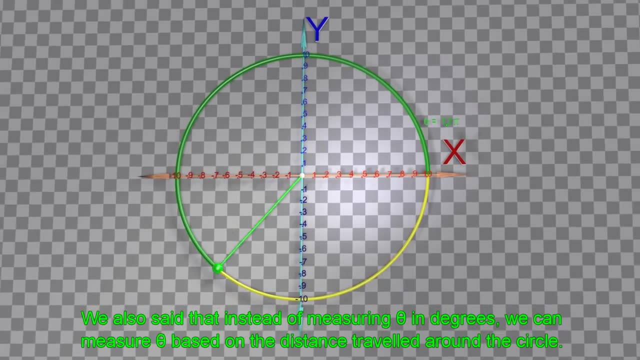 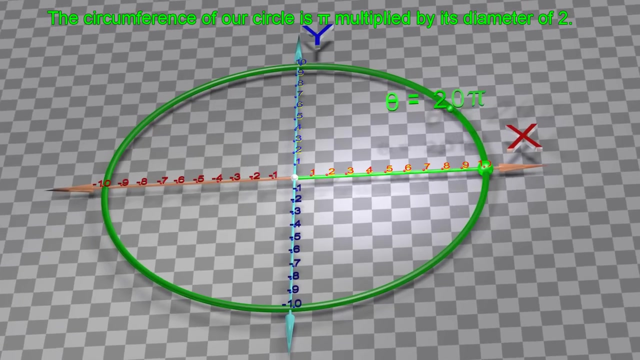 We also said that, instead of measuring theta in degrees, we can measure theta based on the angle. We also said that, instead of measuring theta in degrees, we can measure theta based on the distance traveled around the circle. The circumference of our circle is pi multiplied by its diameter of 2.. 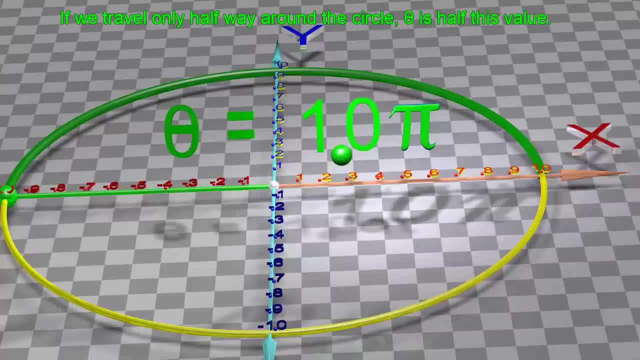 If we travel only halfway around the circle, theta is half this value. This is just to predict the angle that theta will be negative. If we go around the circle in the clockwise direction, theta will be negative In 두� ner. when we are not seeing a point, only a point, is called normal. 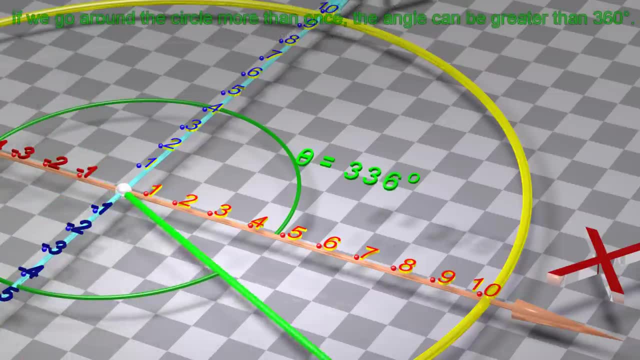 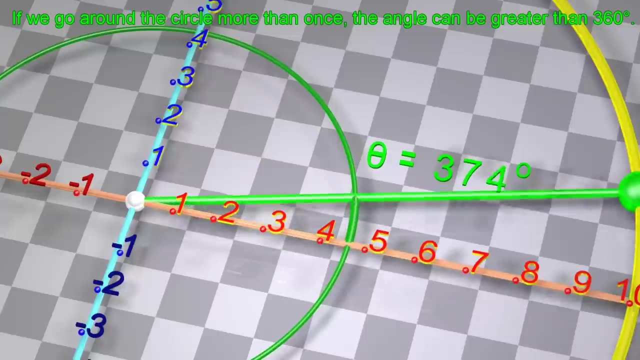 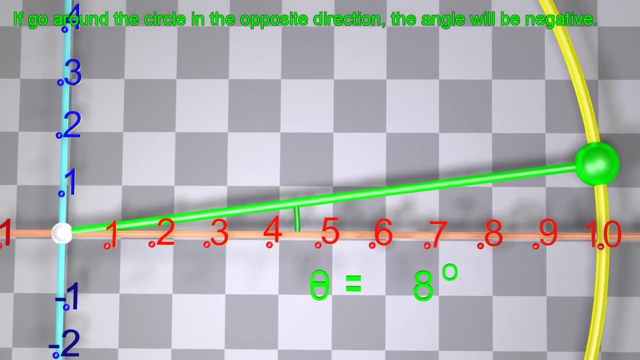 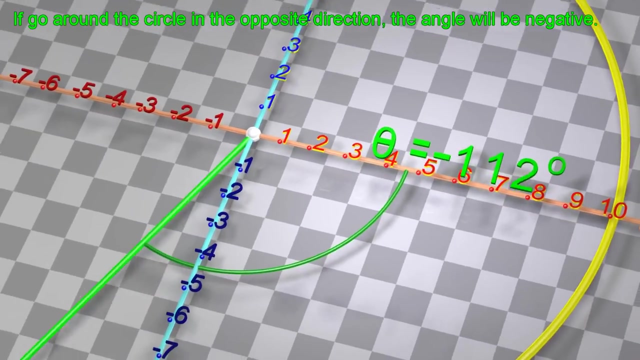 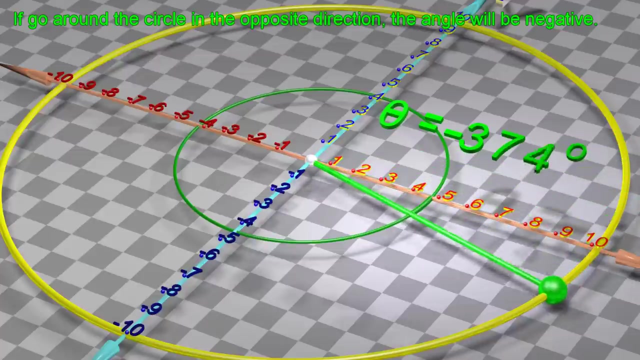 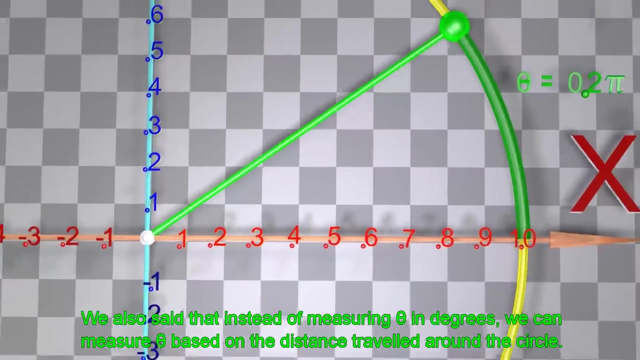 If we go around the circle more than once, the angle can be greater than 360 degrees. If we go around the circle in the opposite direction, the angle will be negative. We also said that, instead of measuring theta in degrees, we can measure theta based on the distance traveled around the circle. 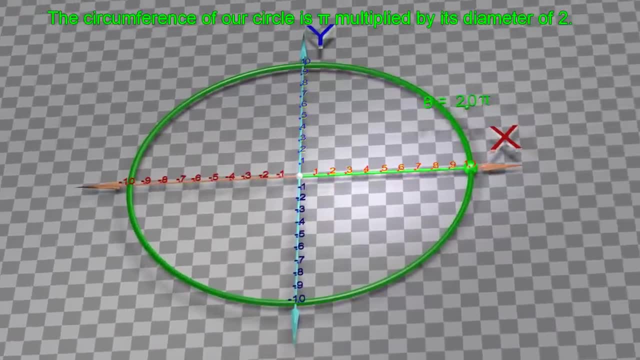 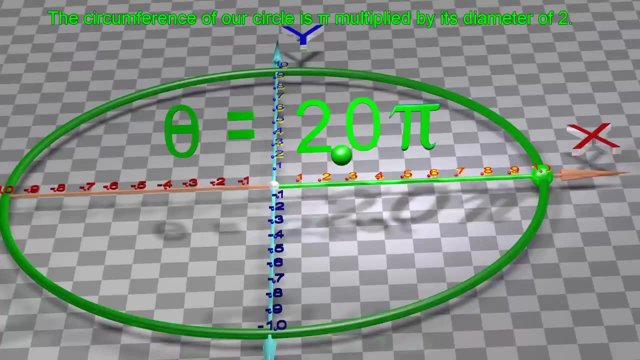 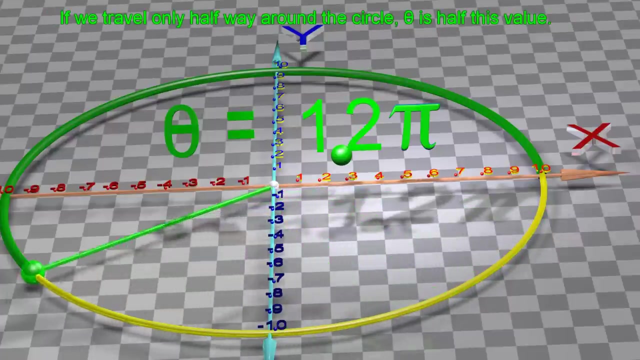 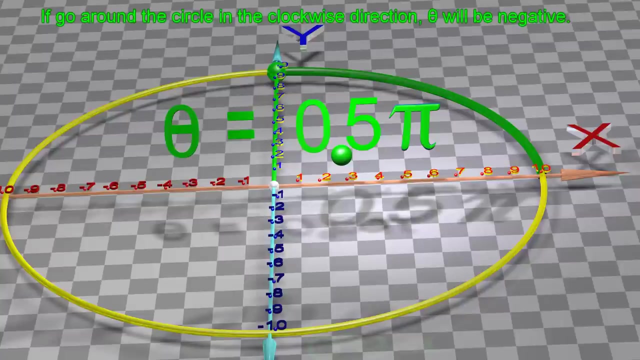 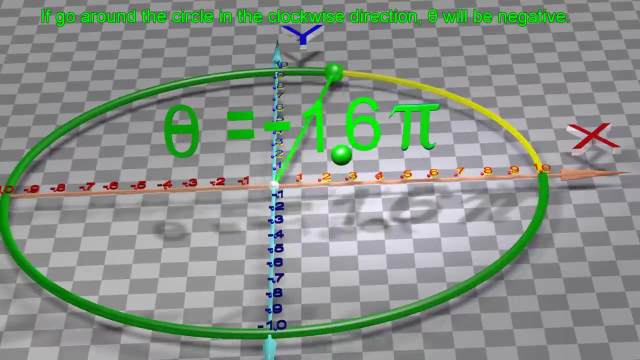 The circumference of our circle is pi multiplied by its diameter of 2.. If we travel only halfway around the circle, theta is half this value. If we go around the circle in the clockwise direction, theta will be negative. If we go around the circle in the clockwise direction, theta will be negative. 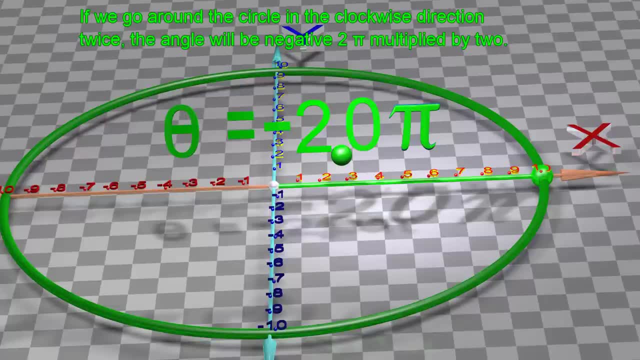 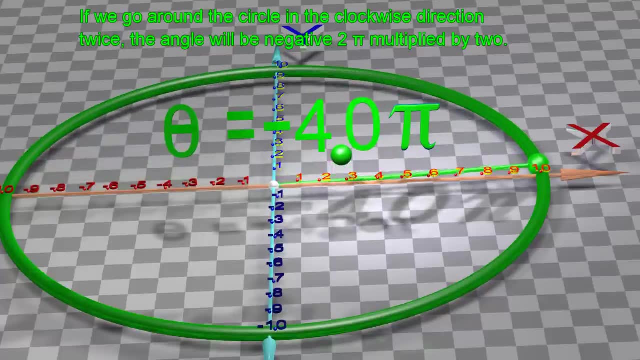 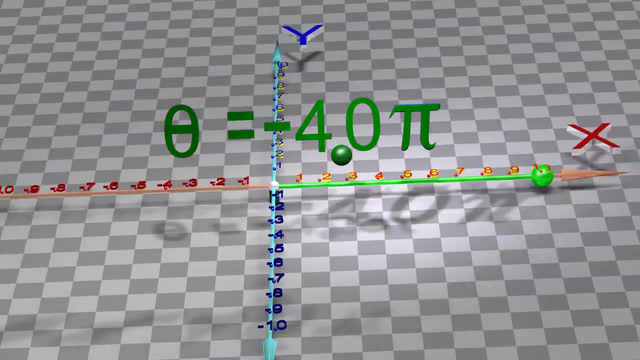 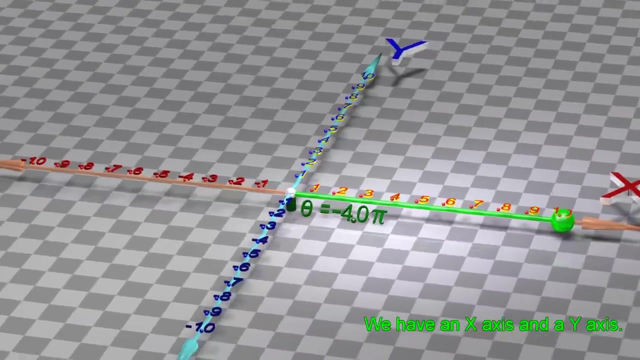 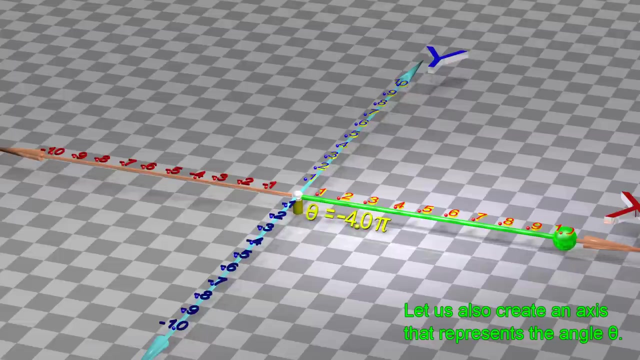 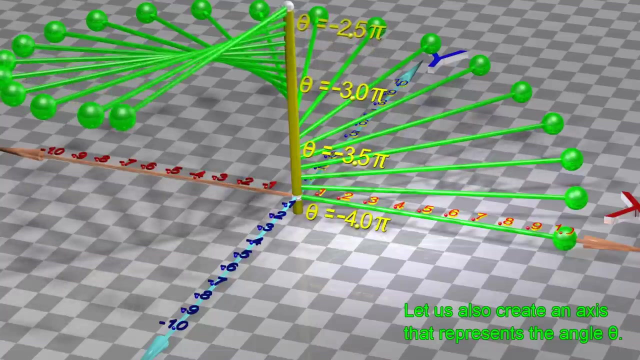 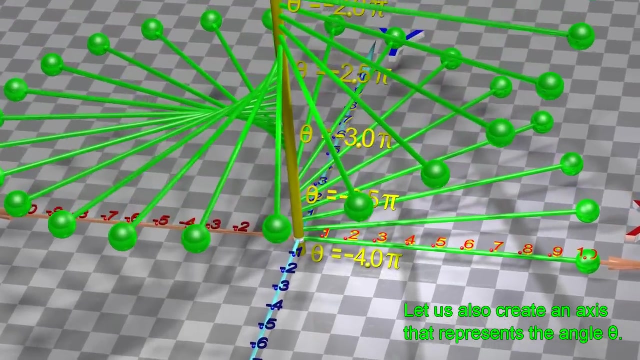 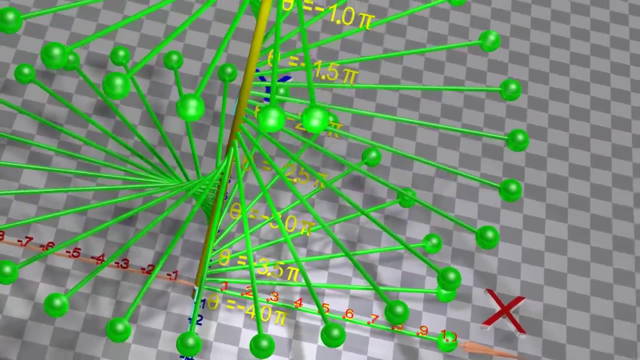 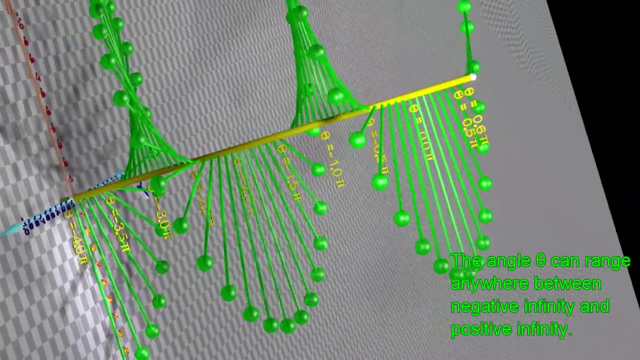 If we go around the circle in the clockwise direction twice, the angle will be negative: 2 pi multiplied by 2.. We have an x-axis and a y-axis. Let us also create an axis that represents the angle theta. The angle theta can range anywhere between negative infinity and positive infinity. 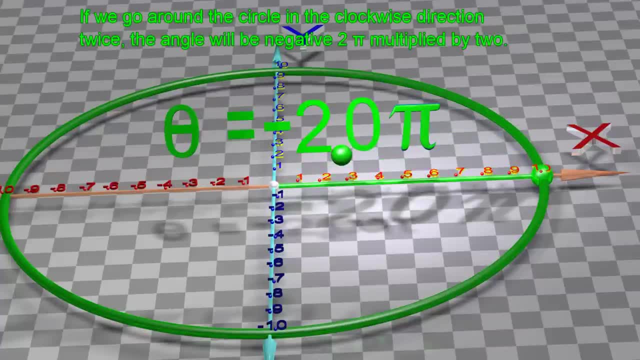 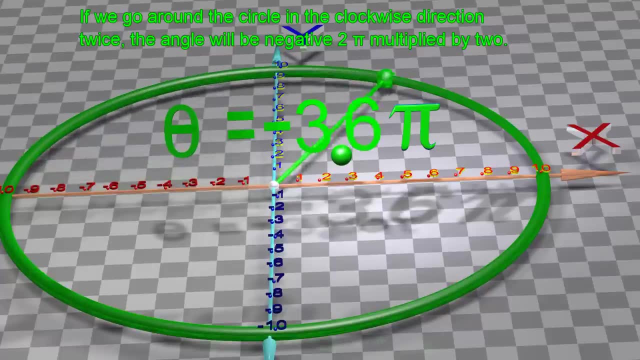 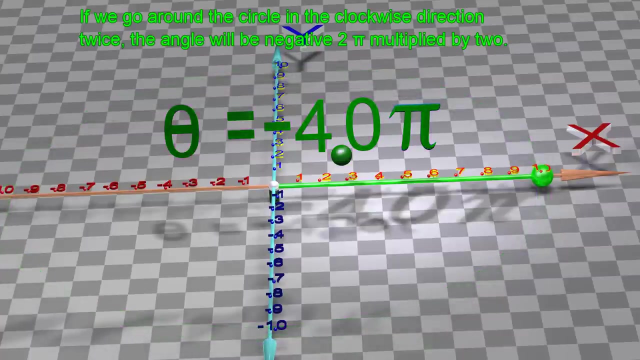 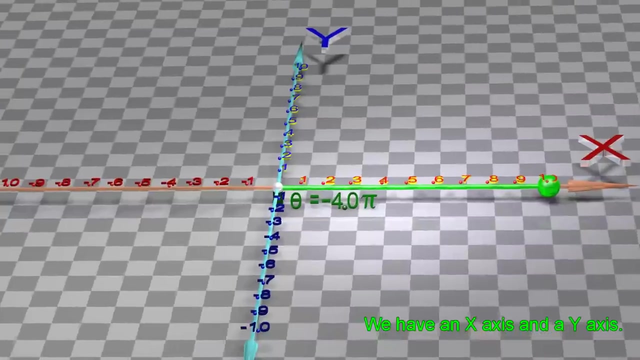 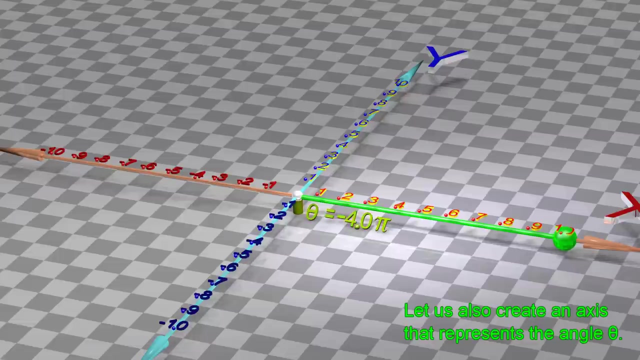 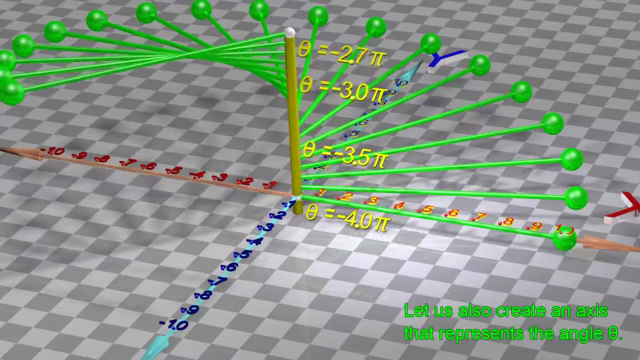 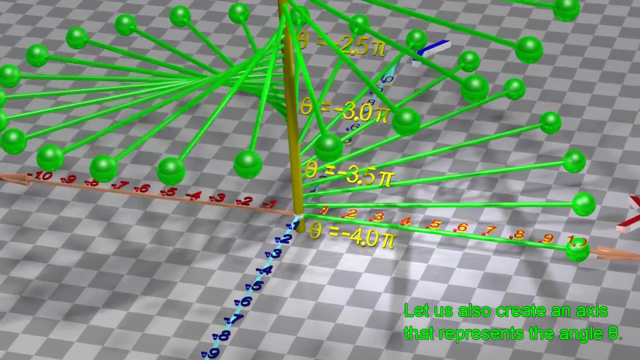 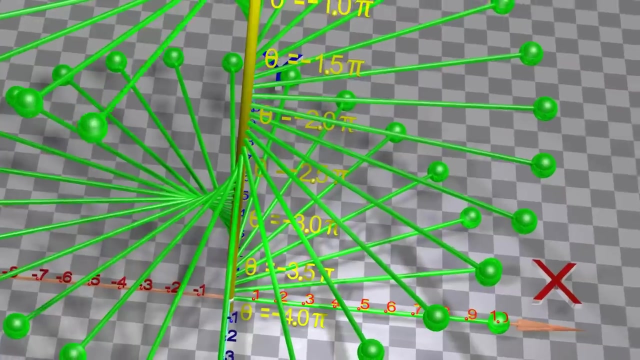 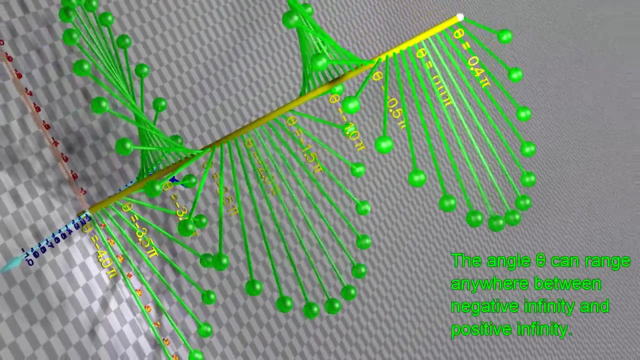 If we go around the circle in the clockwise direction twice, the angle will be negative. two pi multiplied by two, We have an x-axis and a y-axis. Let us also create an axis that represents the angle theta. The angle theta can range anywhere between negative infinity and positive infinity. 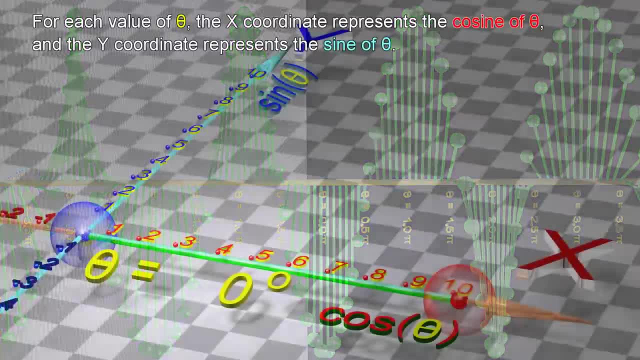 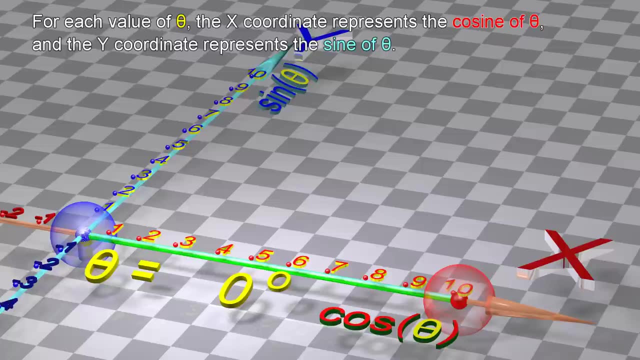 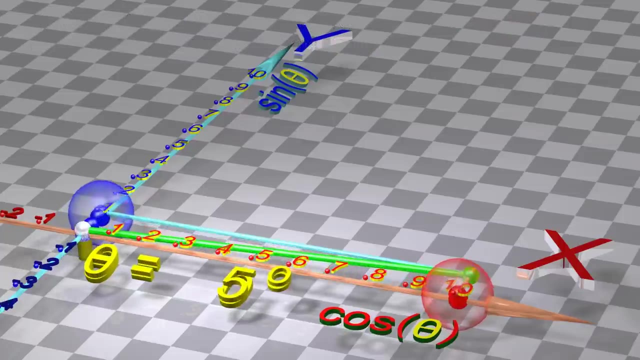 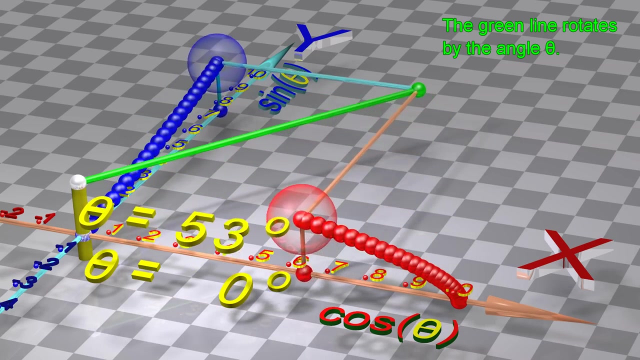 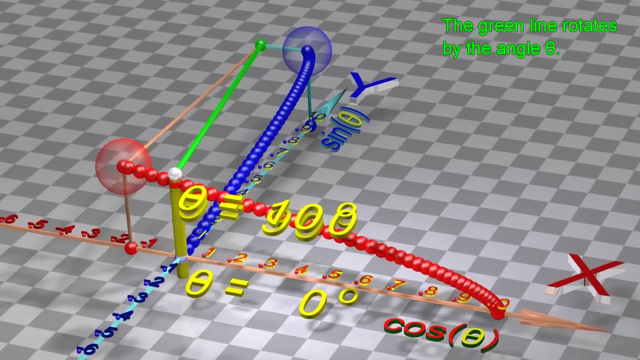 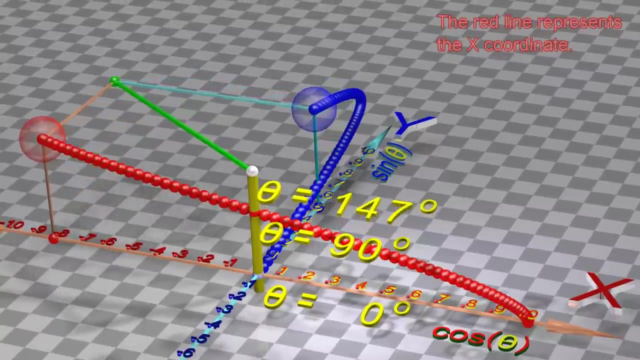 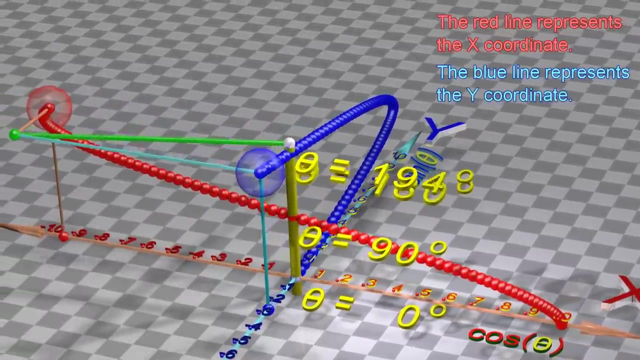 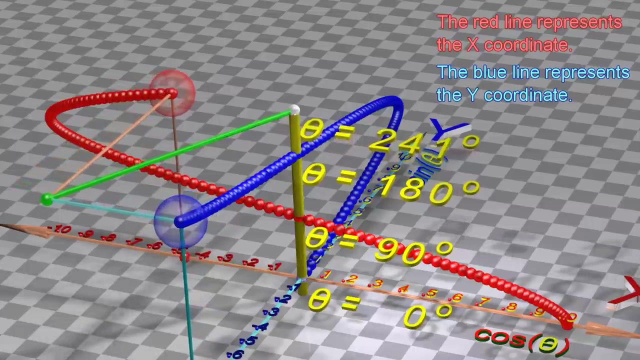 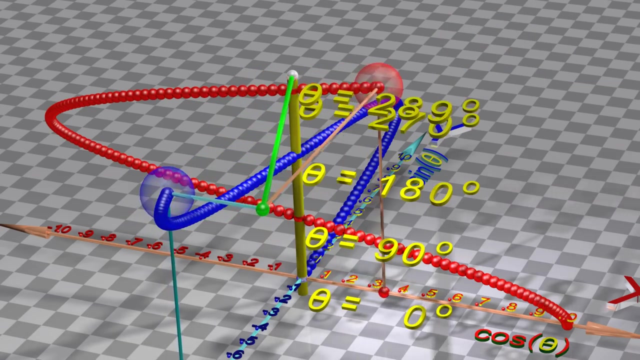 For each value of theta. the x-coordinate represents the cosine of theta and the y-coordinate represents the sine of theta. The green line rotates by the angle theta. The red line represents the x-coordinate, The blue line represents the y-coordinate, The green lines represent the point of contact of the axis. 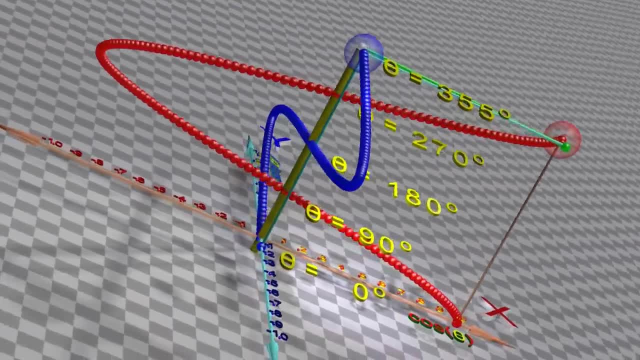 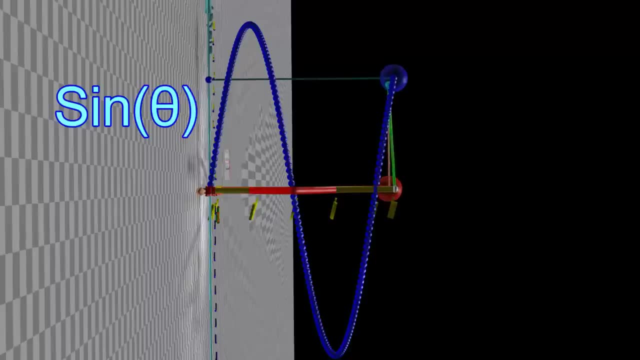 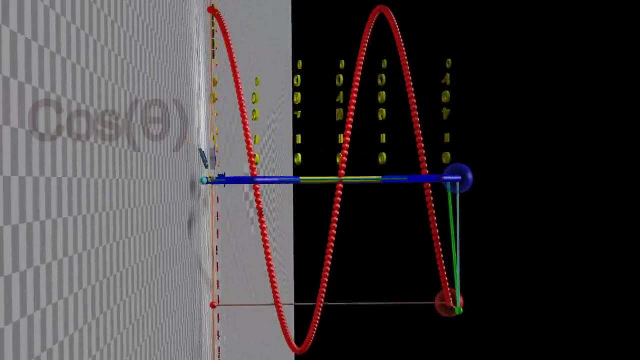 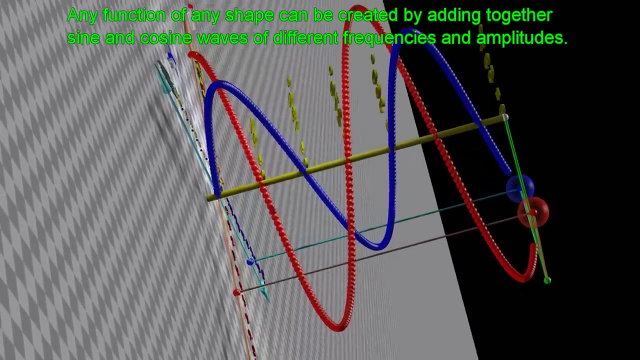 The racing axis represents the axis, The y-axis represents the y-axis and the opposite and acting y-axis. The red line represents the direction of the axis. The x-axis is the position of the x-axis. Any function of any shape can be created by adding together sine and cosine waves of different. 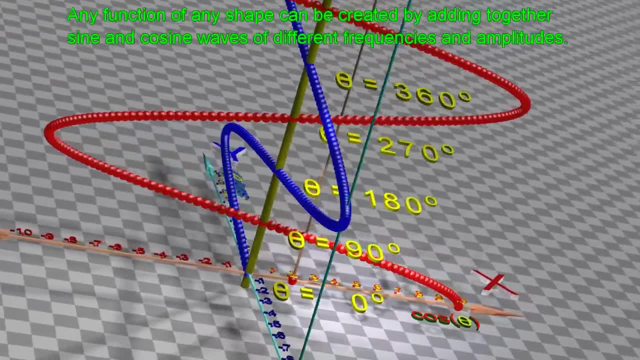 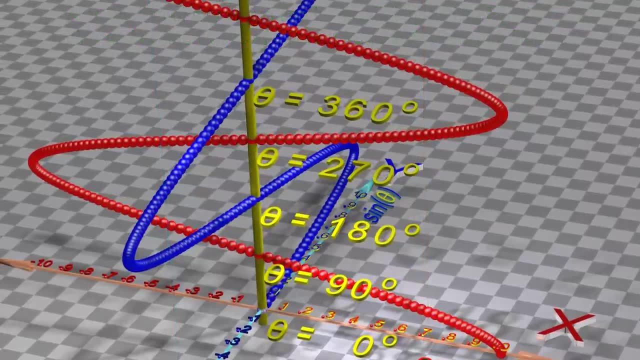 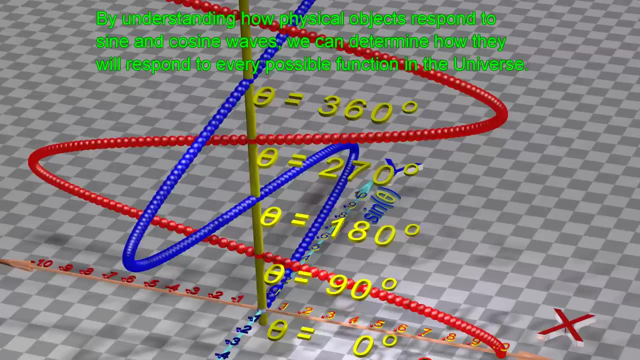 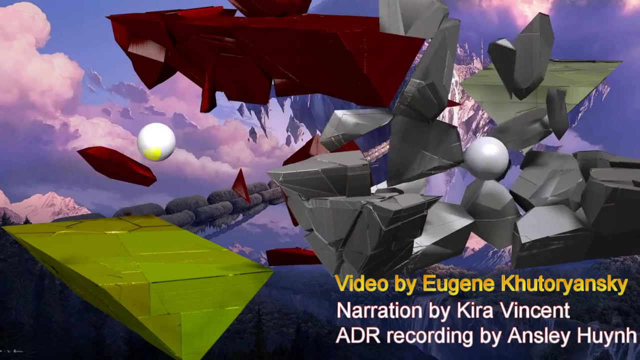 frequencies and amplitudes. By understanding how physical objects respond to sine and cosine waves, we can determine how they will respond to every possible function in the Universe. Subtitles by the Amaraorg community. 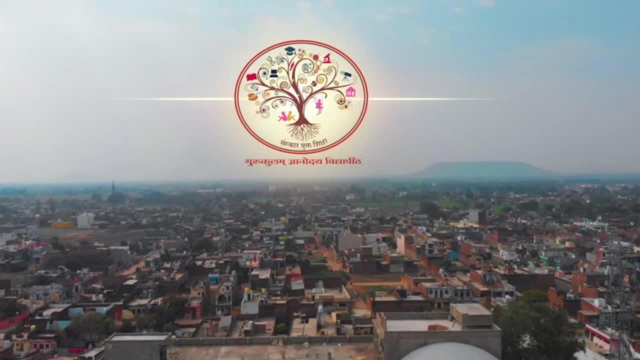 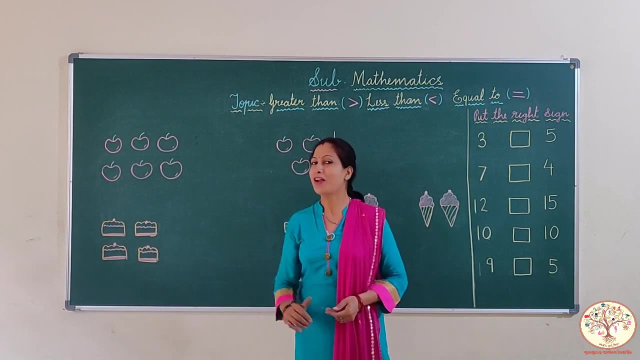 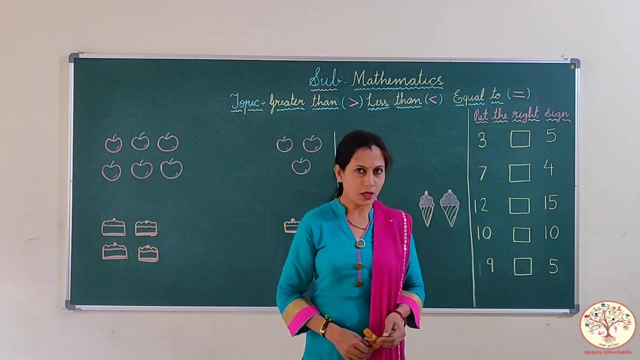 Hello, dear kids, this is Himanshi from Gurukulam Jnana, Vidyavidya Peet. Welcome once again to our mathematics class Kids. today I am telling you a story Story of Cuckoo. Cuckoo the Crocodile. 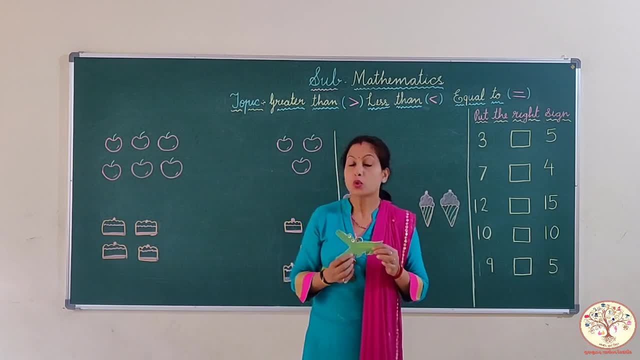 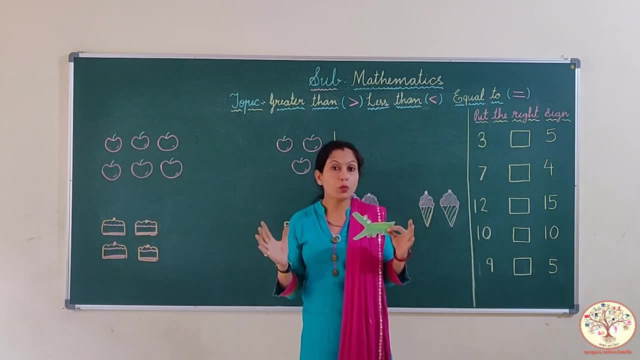 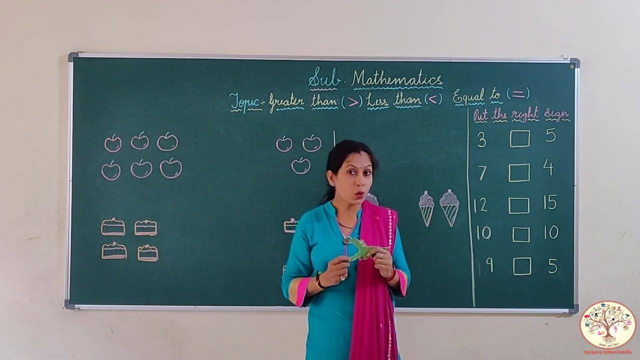 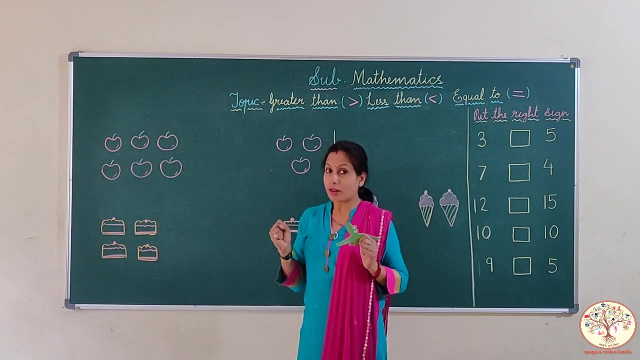 What is its name? Cuckoo Crocodile. So Cuckoo remains always hungry. Cuckoo always used to feel very hungry. When you feel hungry, you eat food, Yes or No? Yes, When I feel hungry, I also tell my mom: Mom, I want to eat a lot of food. 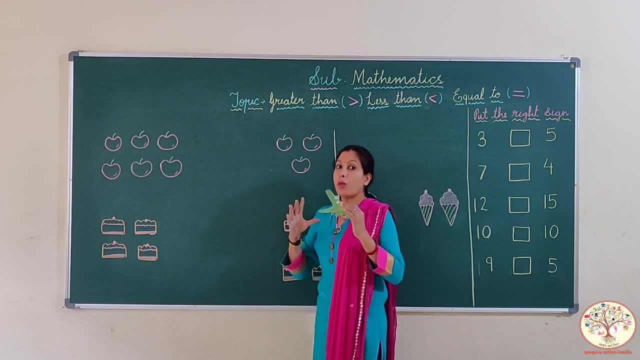 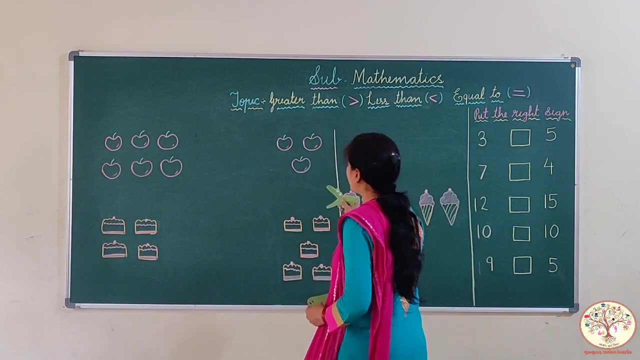 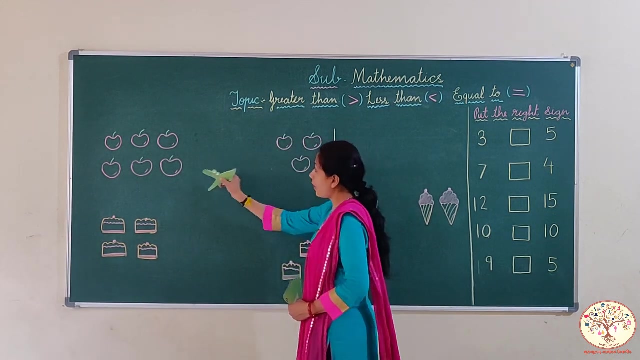 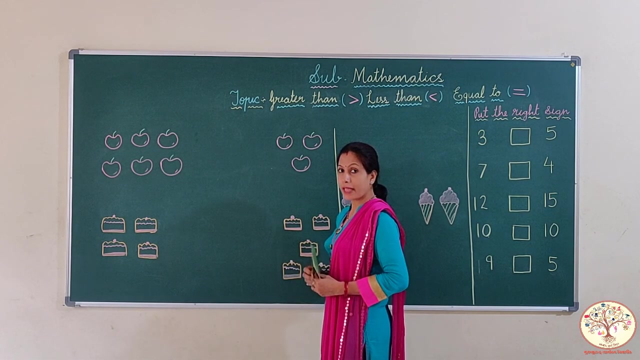 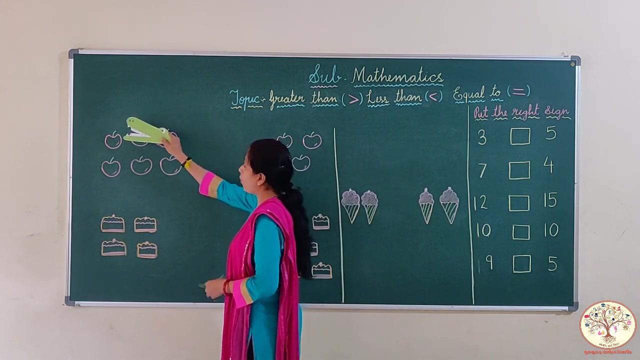 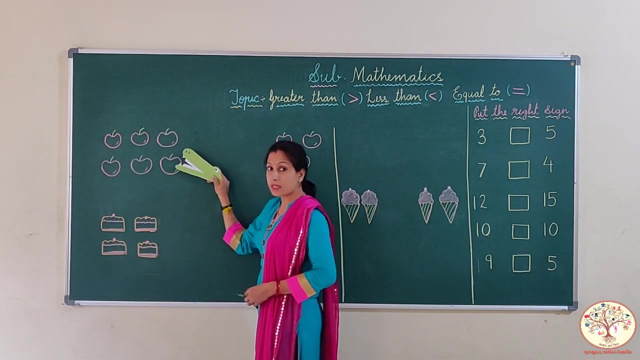 So Cuckoo always eats more food. Ok, So look here, Cuckoo find some apples. there are two groups of apples. which one, which group, has more apples? Can you tell? Ok, let's count One, two, three, four, five, six.